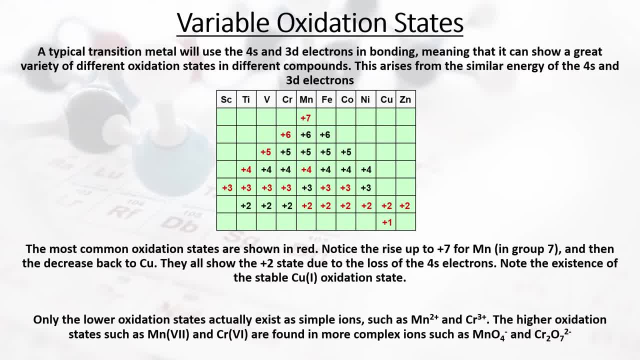 very small number of electrons in bonding. In the first video of this series you might remember that I said that once we take our isolated metal atom or our ion and we then start to put it into the, essentially start to bond it to ligands and put it with other 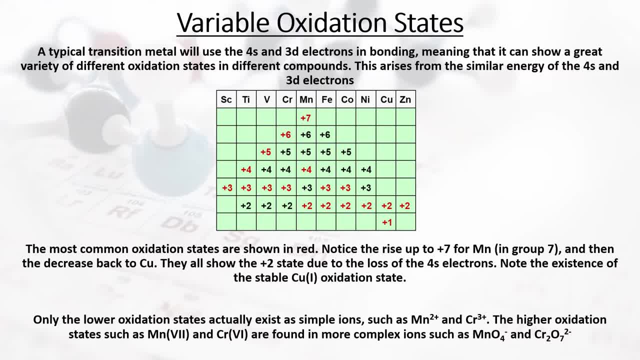 atoms and molecules, But typically our. we normally thought of our 4S level being slightly below the 3D. Typically, when we actually make our molecules and our compounds, the 3D electrons drop slightly below the 4S. Typically we often just think about the 3D electrons drop slightly. 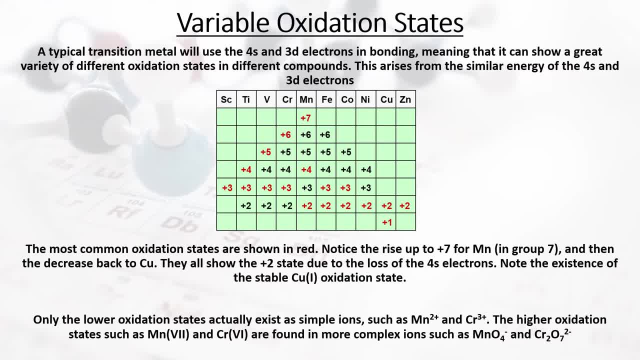 below the 4S, And so that's why we start to make a transition metal atom or a 3D electron to bond it into the 4S. So we're going to look at this transition metal and we're going to about d electrons as being the s and the d in this case, And so because these 4s and 3d electrons 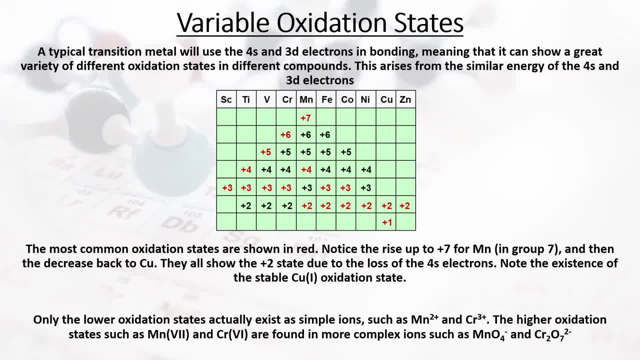 have very, very similar energies. it's very, very easy for electrons to be kind of constantly moved throughout the 3d orbitals and also the 4s orbitals, And so they can show a great variety of different oxidation states in different compounds because of the similar energy of. 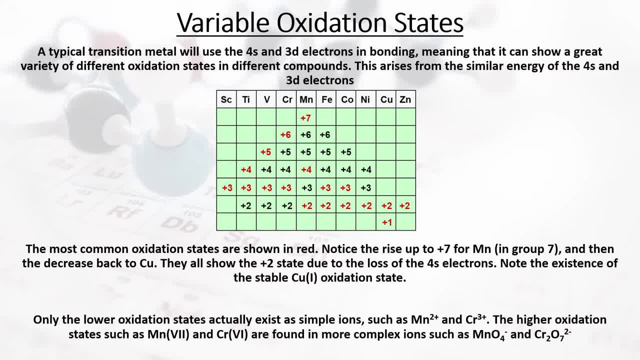 those orbitals because it's so easy to move electrons around, And so you can see this table here of essentially our d block metals. Remember that scandium and zinc typically aren't defined as transition metal ions because the scandium only forms the 3 plus ion, which has a 3d naught. 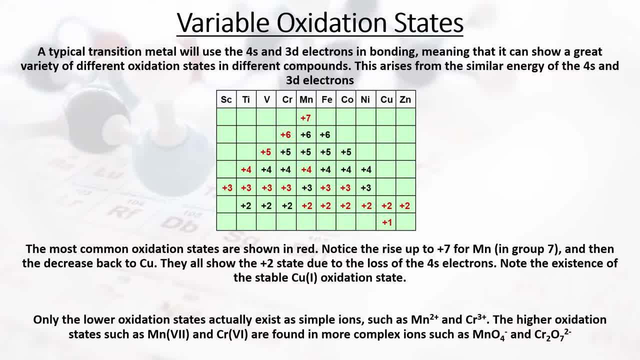 configuration, The zinc only forms the plus 2 stable ion, which makes it a 3d10 system, And so remember that the transition metals had to have this part filled d orbitals. Now, the most common oxidation states for these metals are shown in red And hopefully what you can notice. 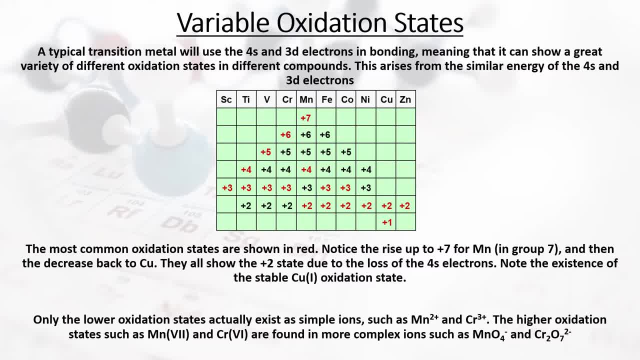 is there's basically a rise. as you go from left to right, from scandium going to manganese, there's this rise, And so you can see that scandium just have plus 3, titanium plus 3 and plus 4, mainly vanadium, plus 3 and plus 5, mainly chromium, plus 3 and plus 6, mainly all the way up to. 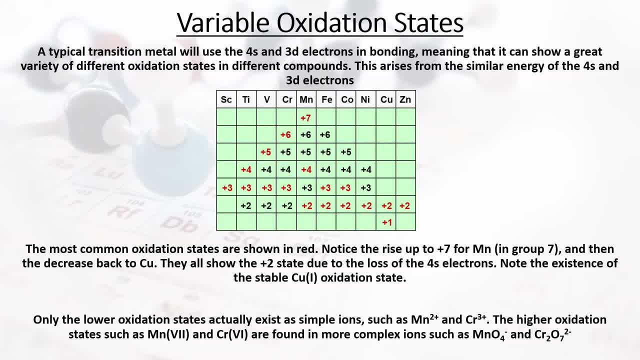 manganese, which often shows plus 2,, plus 4 and plus 7.. But manganese can actually exist anywhere from plus 2 to plus 7.. Vanadium can exist anywhere from plus 2 to plus 5, just the red ones are the. 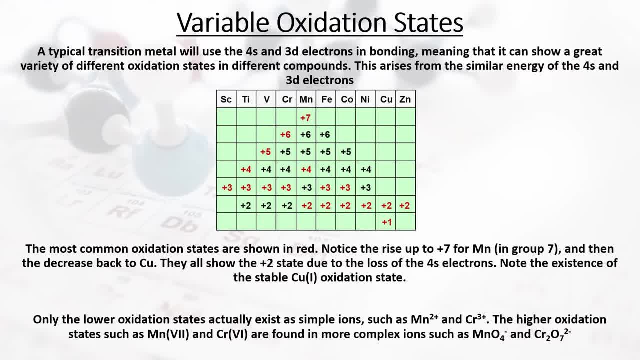 more common that we see. So notice that the red ones are the more common that we see. So notice that there is this increase up to plus 7 for manganese. that's in group 7 of the periodic table And you can see that as you go from the middle there back down to zinc. that essentially we 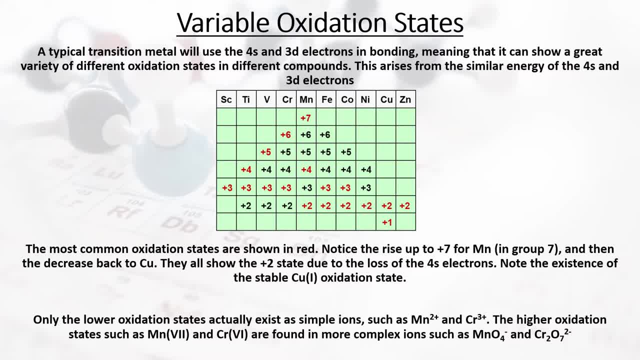 decrease in the maximum oxidation state we can reach. So iron is then down to plus 6 as a maximum, cobalt plus 5, nickel plus 4. And so you can see that generally it drops back down to having just the kind of plus 2 oxidation state for the zinc. at the end. Now they all show this plus 2 oxidation. 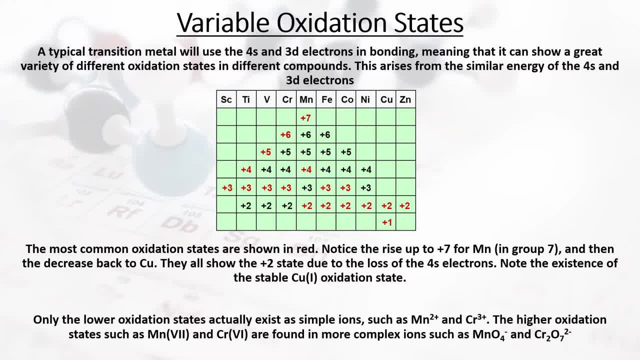 state because, of course, remember that we talked about when the iron oxidates, it's going to be a plus 2 oxidation state. So if we were to ionise our transition metals to make transition metal ions, then it is the 4s electrons that are lost first. And so, because they lose these 4s electrons, 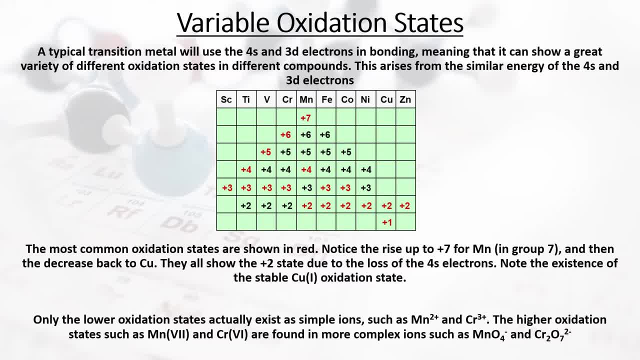 very easily. they all show the plus 2 state. Also note the existence of the only one there that shows a stable plus 1 state is the copper. Copper normally exists either as copper 1 or copper 2.. And now only the lower oxidation states, normally the sort of plus 2 and plus 3 oxidation states. 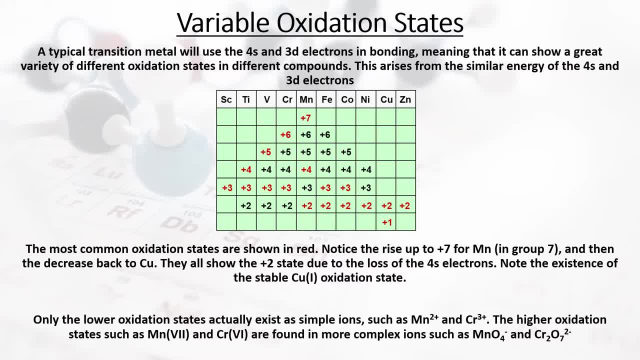 are found to be isolated ions. So for example, the manganese 2 plus ion, the chromium 3 plus ion. these have pretty small oxidation states plus 2 plus 3.. The higher oxidation states, for example the Mn7 or the chromium 6, these much higher oxidation states, aren't found as just isolated. 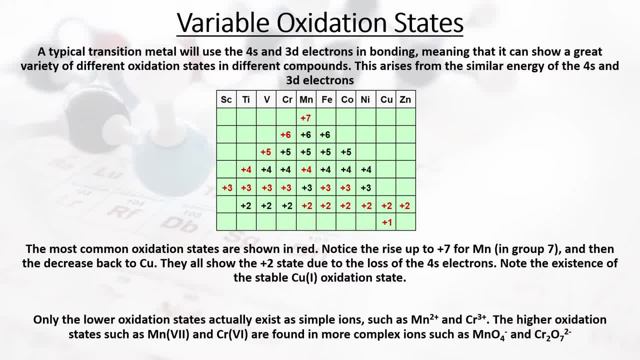 ions. So you don't find the Mn7 plus ion. you don't find the chromium 6 plus ion. What you actually find them in is more complex ions such as the manganate ion MnO4 minus or the chromium. 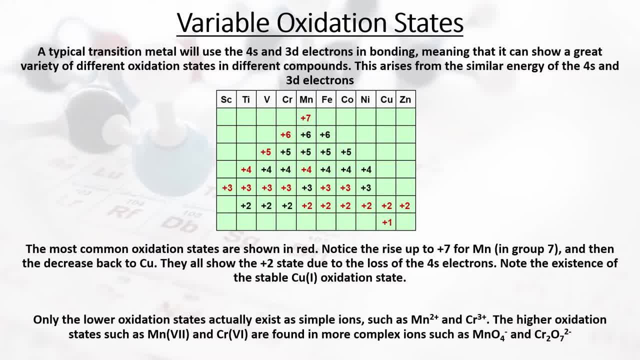 3 plus ion, the dichromate ion Cr2O7, 2 minus, And so if you just kind of review working out oxidation states, you have the MnO4 minus. your oxygen is normally minus 2, 4 of them gives you. 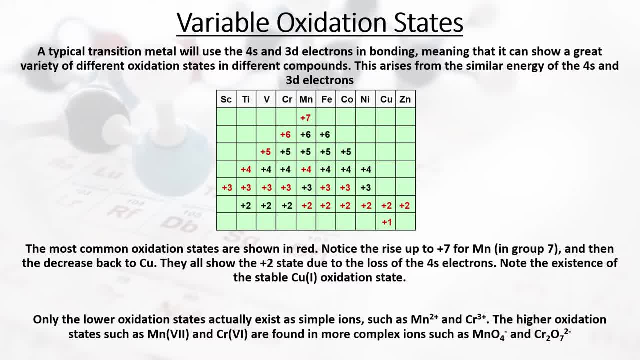 minus 8.. To have a negative charge overall, the manganese must be plus 7, so that's our manganate ion, And then for the dichromate ion we have our oxygen again, normally being minus 2, 7 of them. 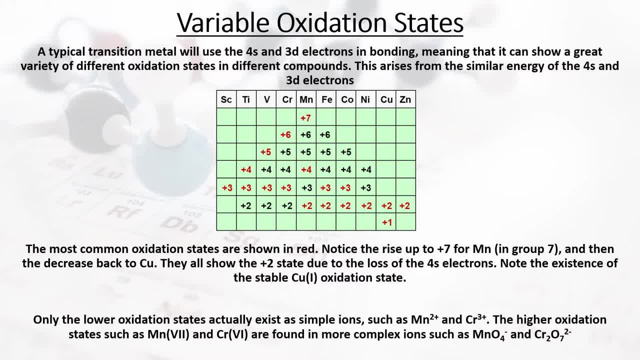 so minus 14.. To have a minus 2 charge overall, each chromium 3 plus ion must be minus 2.. So chromium has to be plus 6 to give plus 12 overall. Now one of the most interesting examples to look. 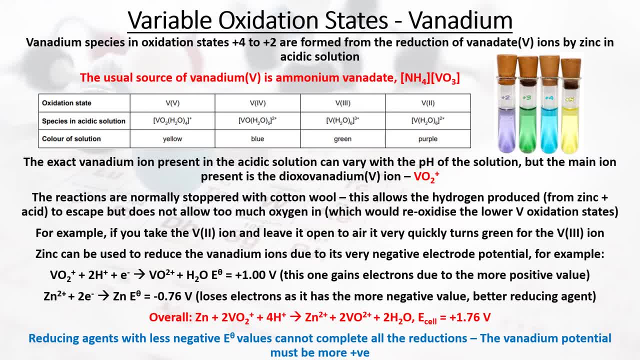 for variable oxidation states is actually to look at vanadium. So we saw for the vanadium that we could take essentially any oxidation state from plus 2 all the way to plus 5.. Now the species in the oxidation states of plus 4 to plus 2 are formed from the reduction of the plus 5 oxidation. 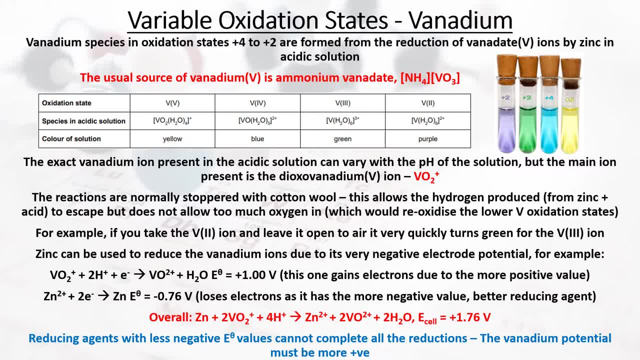 state what we call the vanadate ions, by normally zinc in an acidic solution. So we can reduce our vanadium plus 5 oxidation state to either the 4,, 3, or 2 using zinc in acidic solution And the 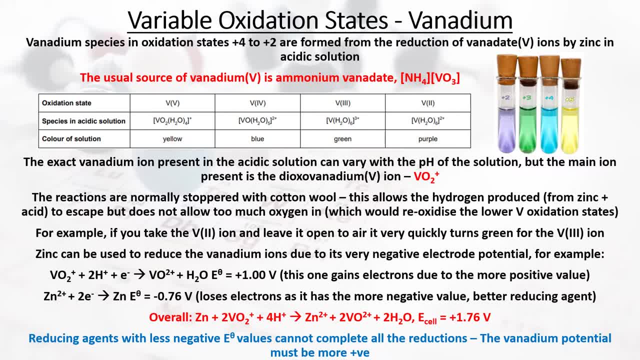 usual source of vanadium 5 is in a compound called ammonium vanadate, That's NH3, 4, VO3.. So if we think about our sort of charges on this, we have our ammonium ion, which is a positive ion. 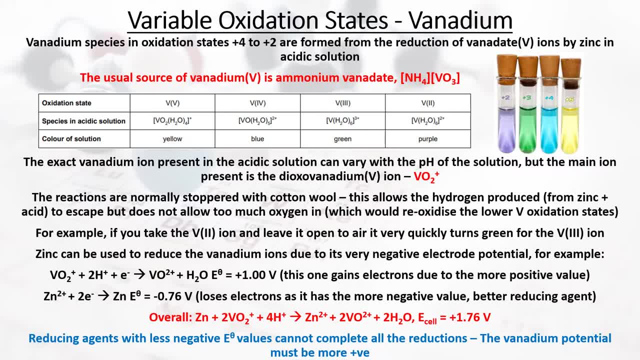 NH4 plus That means back to the overall neutral. our VO3 ion must be overall negative Oxygen, normally minus 2.. So we have three of them to give minus 6. And therefore to give a minus 1 charge. overall the vanadium would be plus 5.. So that's our. 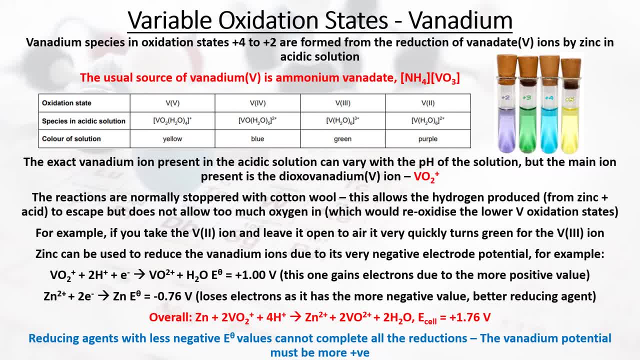 ammonium vanadate, our vanadate ion. And then you can see in this table here I've given you the oxidation states of vanadium from 5 down to 2.. Now you can see here that the vanadium in the 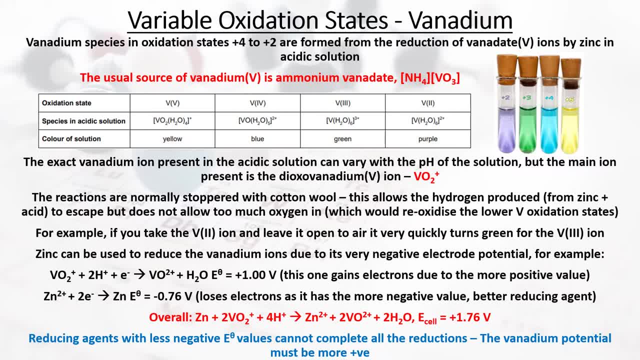 plus 5 oxidation state can also exist as VO3.. So we can see here that the vanadium in the plus 5 oxidation state can also exist as VO2H2O4, plus Now the exact vanadium ion that's present can. 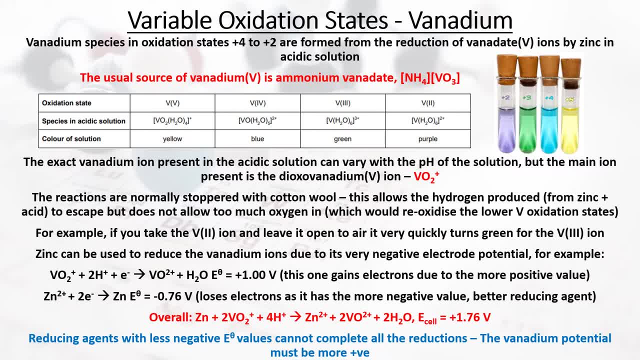 vary with the pH of the solution, It can vary with what the reducing agent that we use is, But typically the main ion is this called the dioxo-vanadium ion. Again, it's vanadium in the plus 5 oxidation state, And so we can find this vanadium either in the ammonium vanadate or as 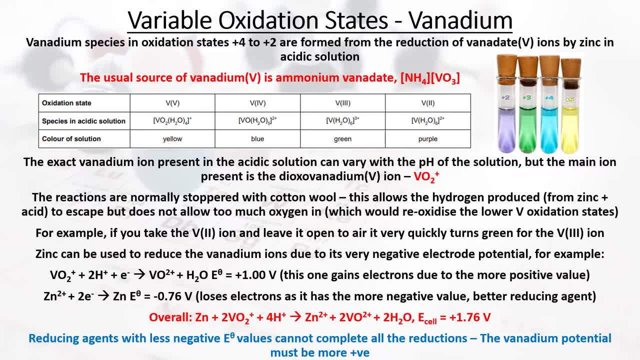 part of this, essentially what was a hexa-aqua ion that's been oxidized? essentially So this VO2 plus ion and then the H2O4, essentially we can think of this as being some sort of aqua ion. Now the actual color of that vanadium in the plus 5 oxidation state here: 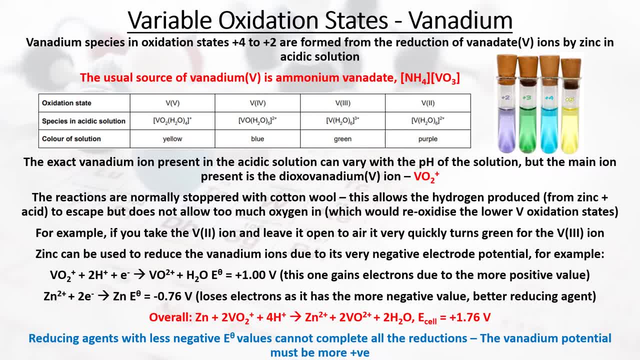 is a yellow color. So what we can imagine is we take our ammonium vanadate, we dissolve it in an acidic solution. This will be typically an aqueous solution, so it has water involved in it. And, like we said back in the first video of this series, if we take a transition metal salt, 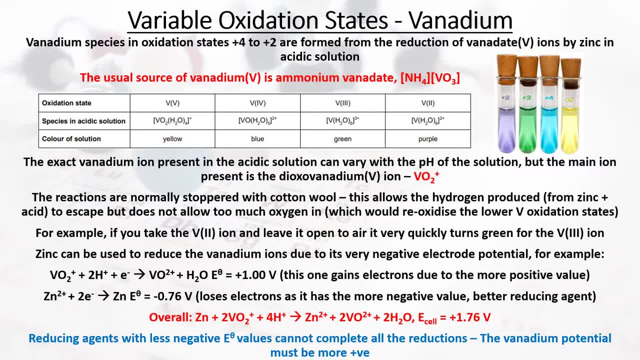 dissolve it up in water. typically, what we actually get is a vanadium in the plus 5 oxidation state. So what we can actually form is our aqua ions. We've talked previously about making things like chromium, iron, hexa-aqua ions- six water molecules. Here we have our vanadium, We have VO2,. 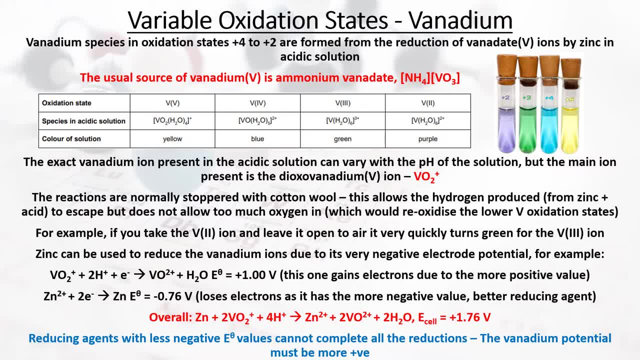 so two of the sites of this octahedral complex are taken up by oxygens, And so therefore we can only fit four water molecules around. So you essentially have a tetra-aqua ion, And so this vanadium, 5 VO2, H2O4 plus is our yellow color. Now we can, as I said, 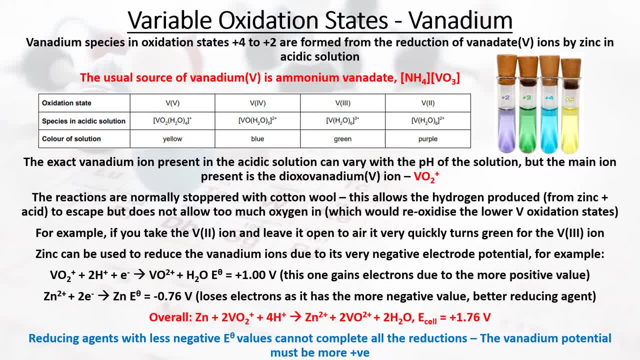 reduce this with our zinc in acidic solution And we can actually reduce it down to the plus 4 oxidation state. This exists as VO H2O5, 2 plus. So you can see, all we've done here essentially is we've lost one of those oxygens from the VO2, and we've added a water molecule, So we've lost one. 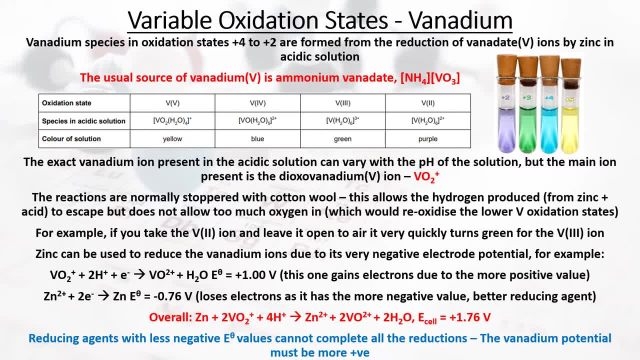 of those oxygens, We can think of it being reduced because we've lost oxygen And so this ends up now being a blue ion. So the color of the solution is blue, And it's important here not to get confused with the actual ions that exist. So if you take away the waters and just consider them as the kind of 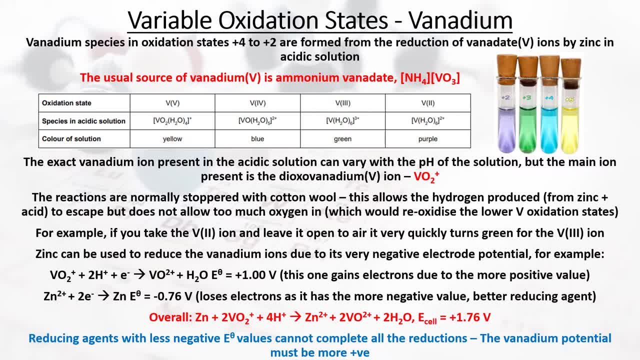 simple ions. in the plus 5 oxidation state, you have the VO2, singly positive ion, The vanadium. in the plus 4 oxidation state, this blue solution, you have the VO2 plus ion. So make sure you know whether it's a 2 plus charge or a VO2 plus 1 charge. essentially, We can then keep on going. 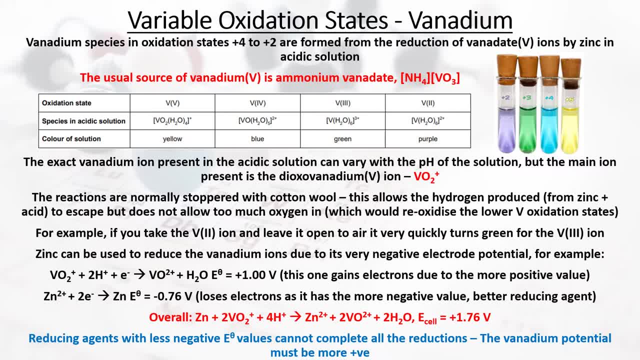 and get all the way down to the vanadium 3 oxidation state. Here we just have the very simple vanadium 3 plus ion V3 plus, And again we can think about our reduction here as a loss of our oxygen. And so we've lost that oxygen from the VO ion to become 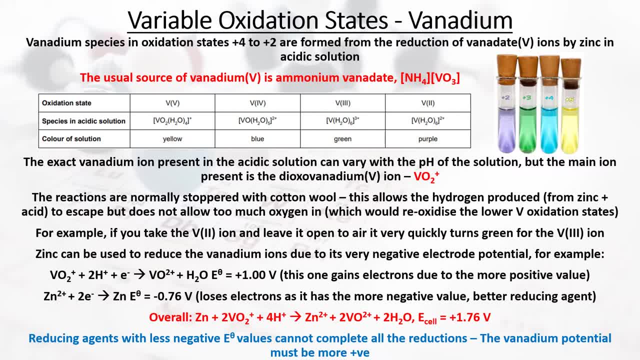 just V. And now we have our vanadium hexa-aqua ion. That's green, And then we can go all the way down to the lowest oxidation state, the vanadium 2.. And this again is a hexa-aqua ion. 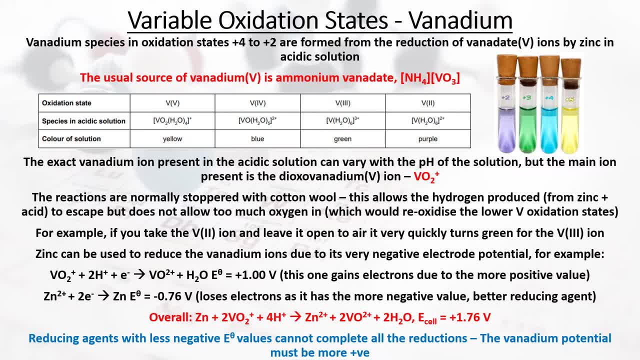 but now it's a 2 plus ion, not a 3 plus ion, And the 3 plus is green, The 2 plus is purple. Now, when we do these reactions, we normally stop them with some cotton wool And this allows the hydrogen that's produced. and the hydrogen gets produced from the reaction between 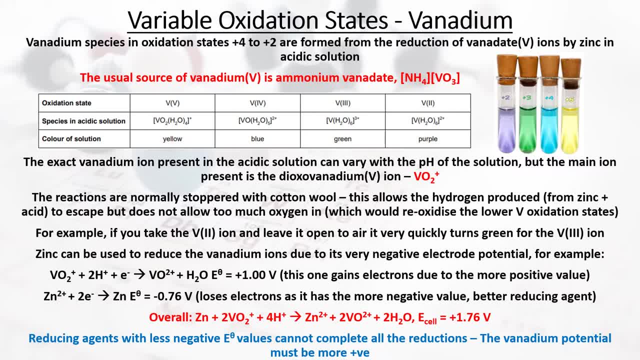 the zinc and the acid that normally ends up producing some sort of zinc salt, some sort of hydrated zinc salt, and hydrogen gas. The cotton wool allows this hydrogen gas to escape. If we just stopped it with a normal sort of full-on stopper, you'd have a buildup. 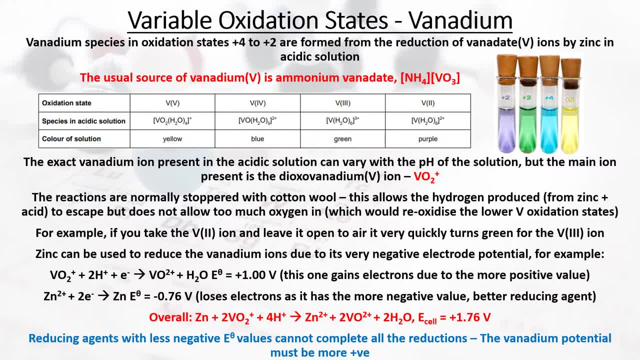 of pressure and that would be dangerous. So we use the cotton wool that allows this hydrogen gas to escape. But if we didn't allow too much oxygen in? and the key thing for this is that if we allow our oxygen in, this would re-oxidise the lower vanadium oxidation state. So let's say we've 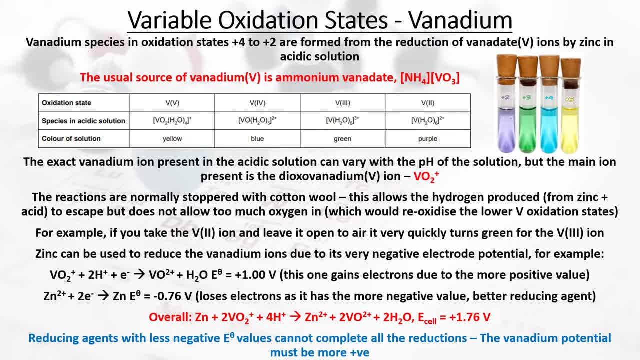 got all the way down to our V2 plus oxidation state, our 2 plus vanadium oxidation state. With that back stopper in there the hydrogen can escape but also the oxygen can get in and oxidise it, potentially all the way back up to that vanadium plus five. And so if you 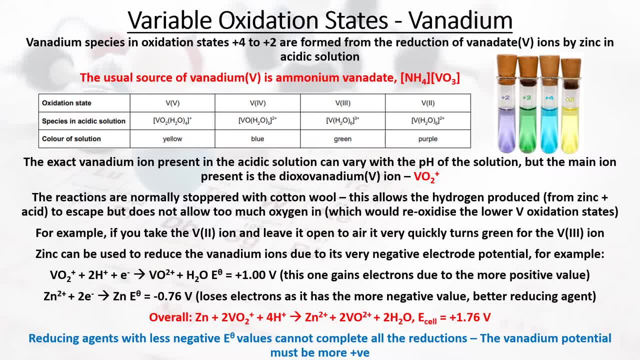 take the V2 plus ion and leave it open to air, it very quickly goes from looking purple to green V3 plus ion. Now the reason that we use zinc actually goes back to thinking about electrode potentials and electrochemistry. So if you're not feeling so confident on your electrochemistry, you 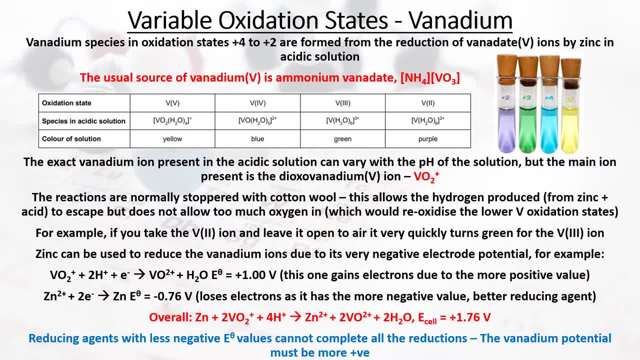 can go back to my series of videos on electrochemistry and electrochemical reactions, But the key thing is that zinc has a very negative electrode potential. What we mean by that is it's a very good reducing agent. It's very good at losing electrons itself and therefore reducing. 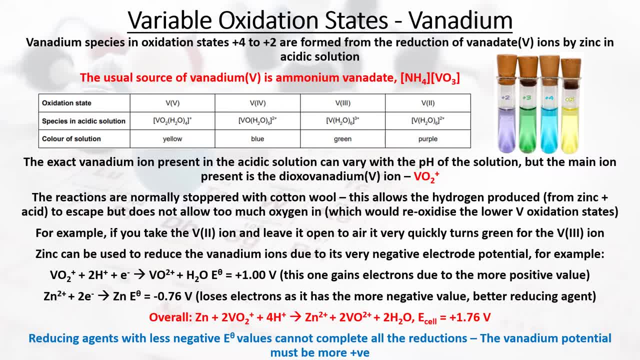 something else. So what do we want to do? We want to reduce our vanadium. So we can think of this in terms of losing our electrons, but also from a more technical point of view. with our redox, We know that from oil rig, oxidation is loss, reduction is gain, And so we want to reduce. 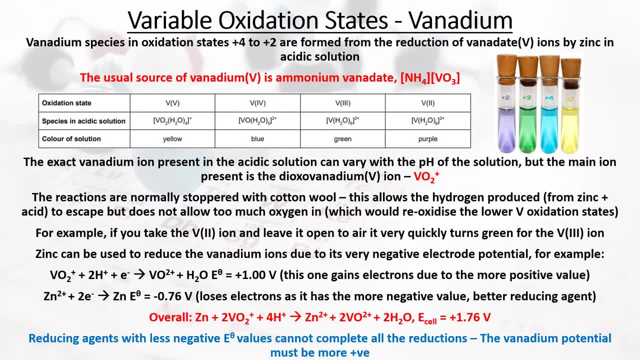 our vanadium by making it gain electrons, And therefore we need something that's a very good reducing agent, something that's very happy to lose electrons, And this turns out that zinc is good for this because it has a very negative electrode potential, And so you can see at the bottom there the zinc electrode potential. Remember these. 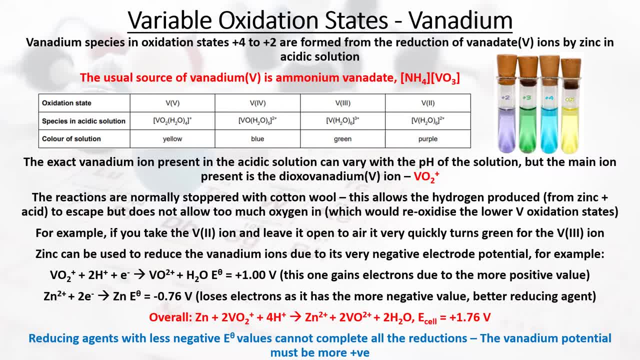 electrode potentials are always written as reductions. So we have our zinc two plus plus two electrons to make the zinc metal. This has this half cell potential of negative 0.76 volts, The actual vanadium equation we have at the top. this is our VO two plus. 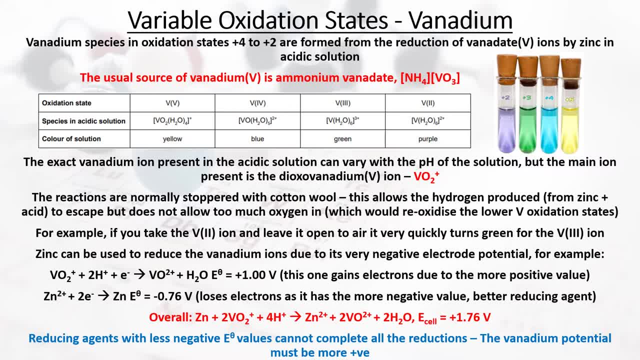 This is our vanadium in the plus five oxidation state Plus two hydrogens plus our electron produces the VO. two plus ion. That's going from the plus five to the plus four oxidation state. That's going from the yellow to the blue solution. And this has a half cell value here of one. 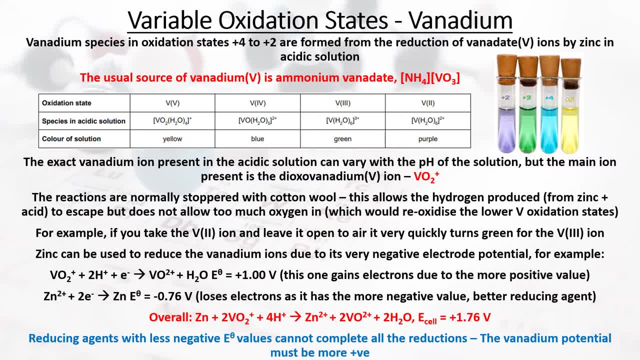 volt plus one volt, And so the way to remember it is always the negative. one loses electrons. It is the one that is actually oxidized. The one that has the more positive value is the one that gains electrons. It's the one that is reduced, So the more positive value gains. 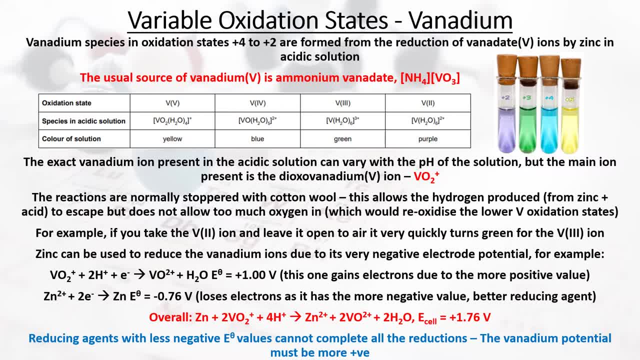 the electrons, The more negative one loses the electrons. It's a better reducing agent. Very simple way that I remember it is that the more negative one is probably going to lose electrons, Because negative repels electrons, Positive attracts electrons. And so if we then essentially our zinc equation, here we need to flip it around the other. 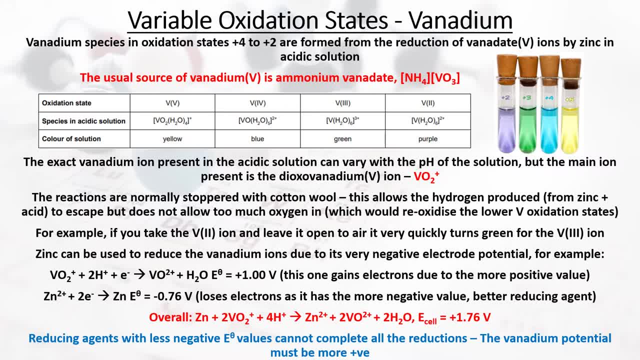 way, because we're having the zinc lose electrons because it's a reducing agent. So we flip the equation around. We multiply that top vanadium equation by two. That will allow us to cancel out our electrons, And when we do that we end up with an overall equation that is zinc plus two of the vanadium. 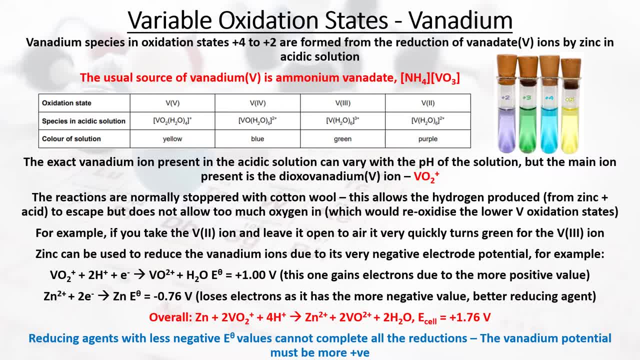 ions. in the plus five oxidation state, the VO2, single positive charge plus four H plus going to zinc, two plus two lots of the vanadium in the plus four oxidation state: the VO2 plus ion and then two lots of water. 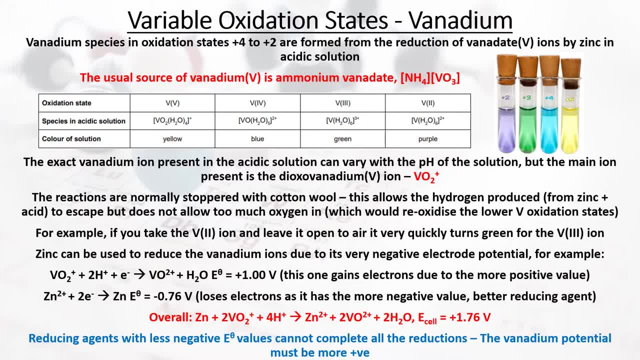 And remember that when we calculate our E cell values we do the cell of the right minus the cell of the left. In this case that means that when we put our numbers in it actually comes out to be positive 1.76.. So quite a high E cell value here. showing this is a very 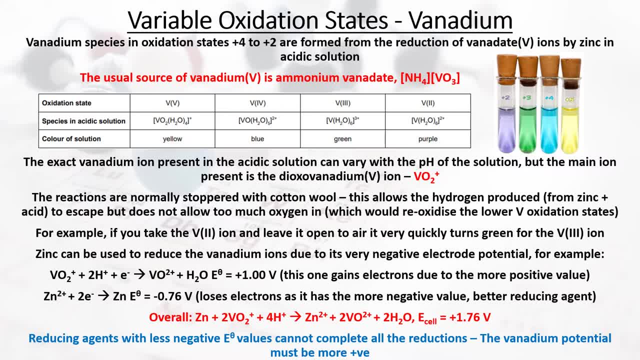 feasible reaction. Now, the reason we use zinc is because, if we have reducing agents that have slightly less negative electropotential values, they can't complete all of the reductions, And so what I've shown you here is essentially the electrochemistry for that first reduction. 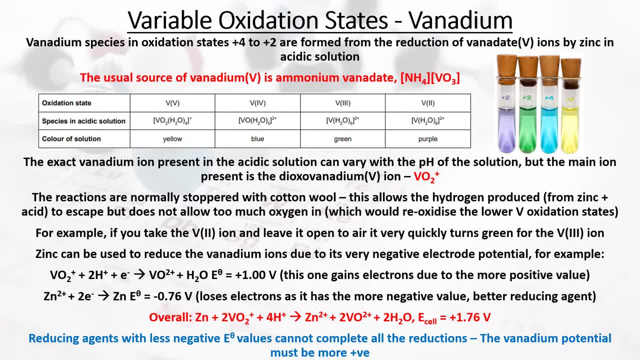 from the plus five to the plus four, But we can think about going all the way down to the plus two ion, And the key thing is that we always need our vanadium potential to be the more positive one. We always want our vanadium to be the one that is being reduced. 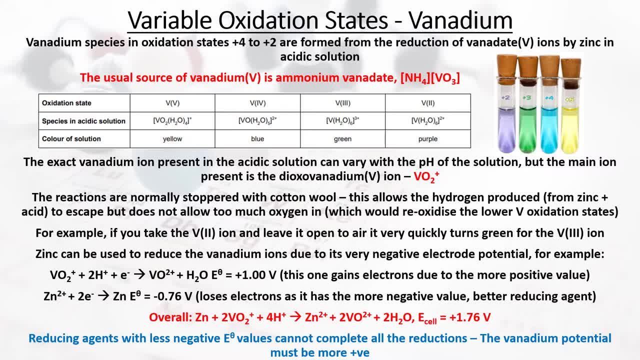 meaning the electrons- For that to happen. the other metal we're using to reduce this, the zinc in this case, has to be more negative in terms of its electropotential. So there are other metals. for example, you can get some of the earlier ones reduced using tin. 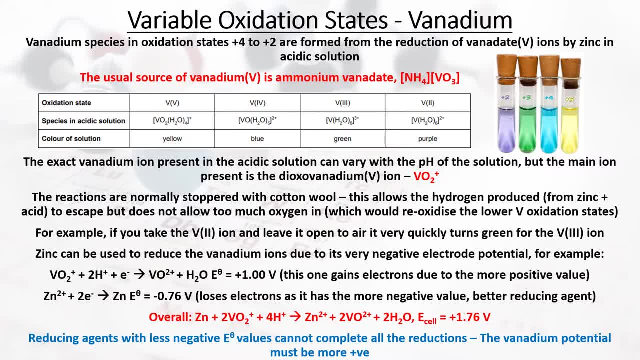 for example in acid solution, But the later ones. tin just simply doesn't have a negative enough electropotential. But there comes a point where the tin has the more positive and the vanadium has the more negative, which is the wrong way around. We always want to. 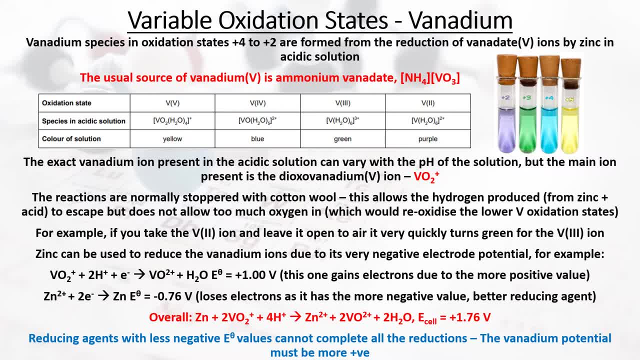 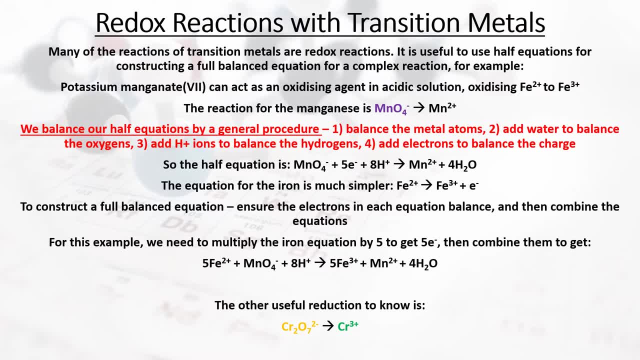 have vanadium potential to be more positive than the other. Now we can think, then, about doing redox reactions with transition metals, And many of the reactions are actually redox reactions, And so it's useful to use half equations for these to see, essentially, whether we're oxidising or reducing, and then being able to construct. 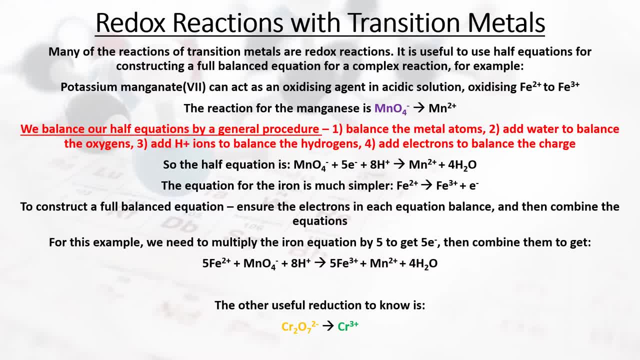 a full, balanced equation. So for example, we have potassium manganate, that's our manganate, seven ions MnO4 minus, And these can act as an oxidising agent in acidic solutions. So for example, it might oxidise Fe2 plus to Fe3 plus. Now again, note here that our reaction to the manganese is: 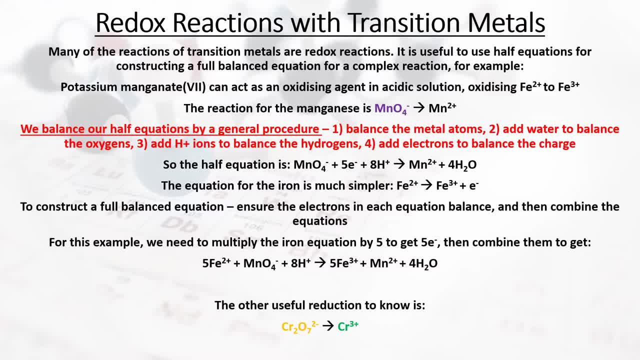 that we have our manganate ion, the manganate seven, MnO4 minus going all the way down to Mn2 plus. And note again here that your lower oxidation state of the Mn2 plus exists as the simple ion. The MnO4 minus actually exists as our complex 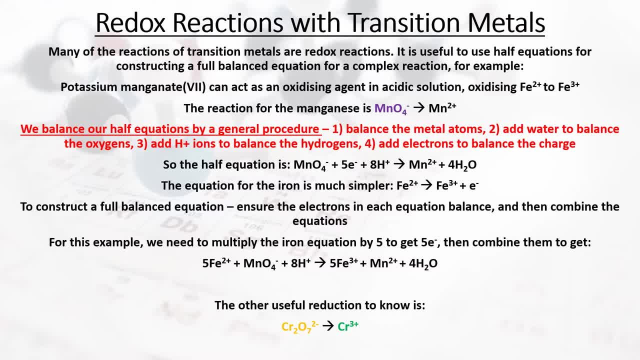 ion essentially So the high oxidation state is bonded to other atoms. So we balance our half equations by a general procedure And this goes back again. if you're not so happy with half equations and redox chemistry, go back to my series of videos. 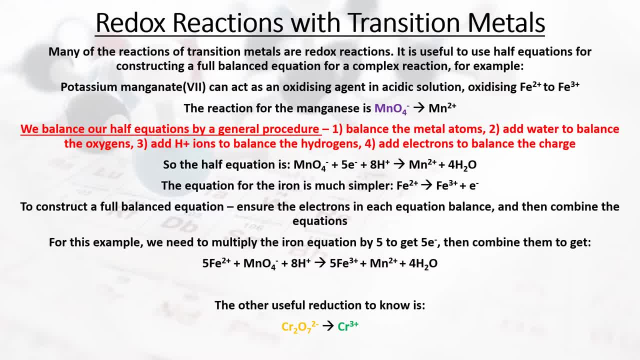 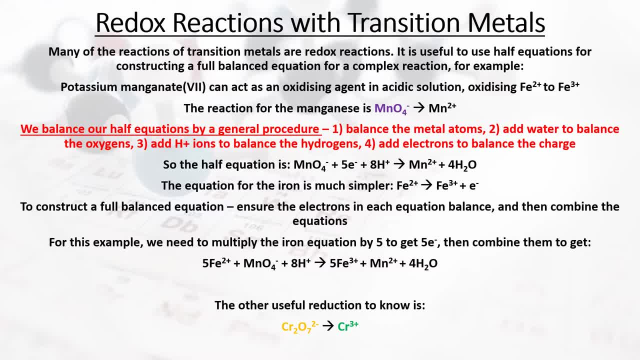 we have to add water to balance the oxygens. Now, if there's no oxygens present, you skip this step. However, we have MnO4 minus, so we have four oxygens on the left-hand side, none on the right. So we have to add four water molecules to balance those oxygens, So 4H2O would go. 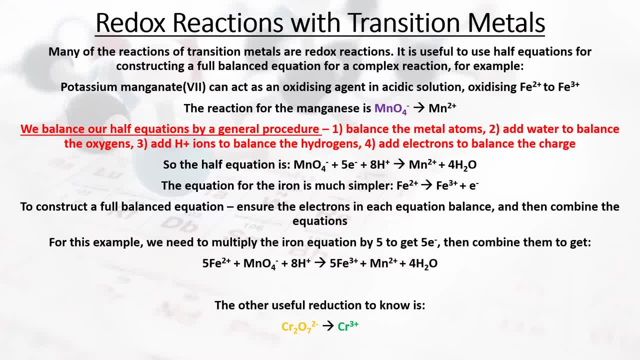 on the right-hand side. Then if you have any hydrogens present- which we do now because we've added water- we have to add H plus ions. This is normally why we do these in acidic solution. In the previous example we have 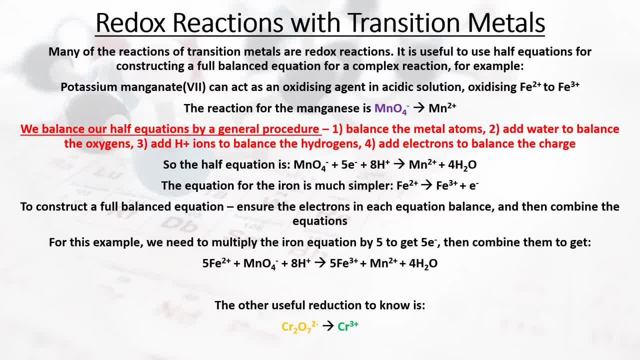 this reduction of the vanadium, The vanadium in acidic zinc solution, And so we add H plus ions to balance out the hydrogens, And so in our case here we added four hydrogens to the right-hand side to balance the oxygens. 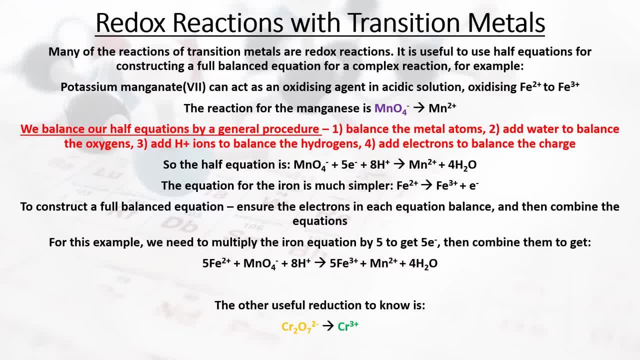 Sorry, we added four water molecules, sorry to balance out the oxygens. Therefore we have eight hydrogen atoms, essentially on the right-hand side. So we have to add eight H plus ions on the left-hand side, And then the final thing to do is to simply add electrons to balance the charge. 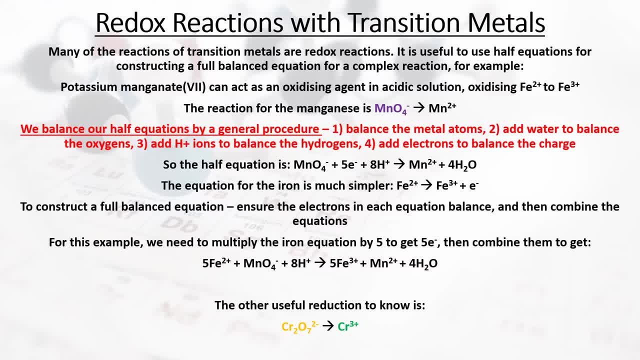 So this is any kind of normal equation. We have to make sure there are atoms in our charge balance on both sides, And so in this case we have a two plus charge on the right-hand side. To get the left-hand side to have the same two plus charge, we have to add five electrons. 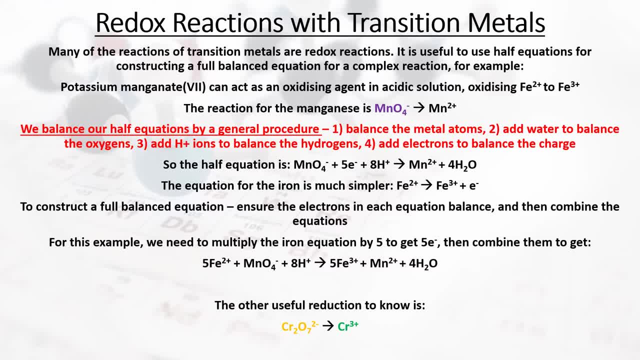 And so our balanced half equation here is MnO4 minus plus five electrons plus eight H plus going to Mn2 plus plus 4H2O. So always follow that general procedure: Balance the metal atoms. If there's any oxygens present, we add H plus ions to balance out the oxygens. 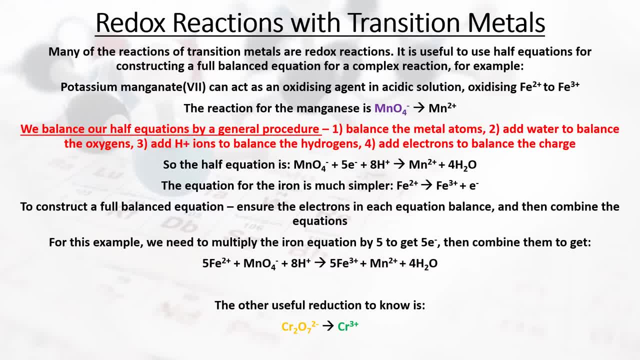 And then we add H plus ions. If there's any hydrogens present, balance it with water. If there's any hydrogens present, balance it with H plus ions And then make sure the charge balances by adding electrons to whatever side needs it. 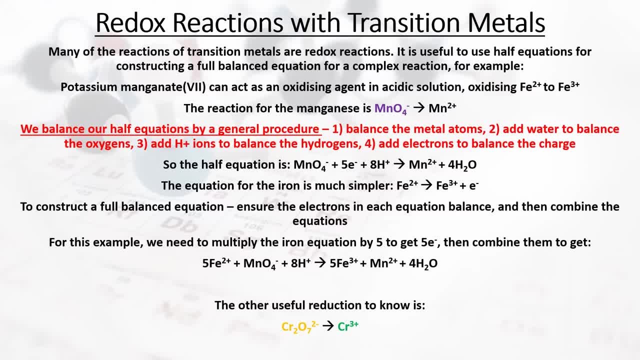 Now the half equation for the other species. here the ion is much, much simpler. We have Fe2 going to Fe3, plus that oxidizes this ion with lost electron, And so our equation just becomes: essentially we don't have to worry about balancing our 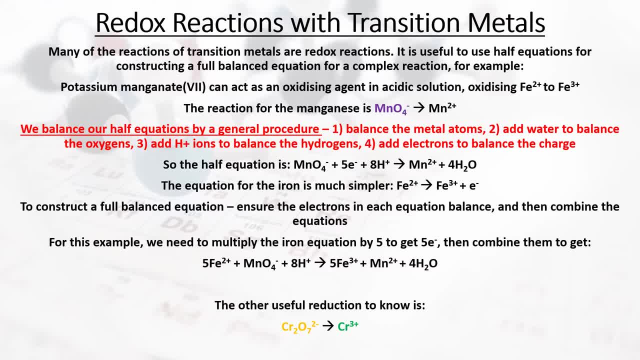 metal atoms. We don't have to worry about adding waters because there's no oxygen. We don't have to worry about adding protons because there's no hydrogen. So all we have to do is balance the charge by adding an electron to the right-hand side. 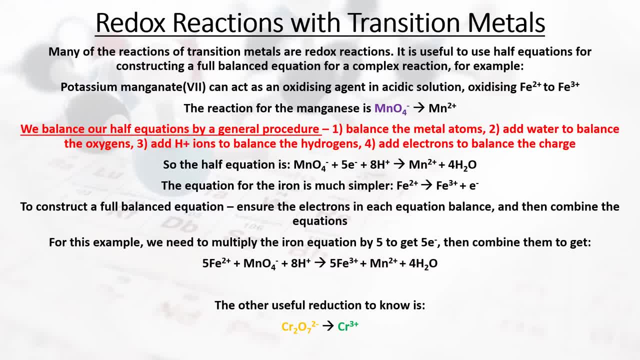 And then to construct our full balanced equation we have to ensure that our electrons in each equation balance, so we have the same numbers of electrons in each equation And then we combine the equations. So you can see here that for the manganese equation we have five electrons. 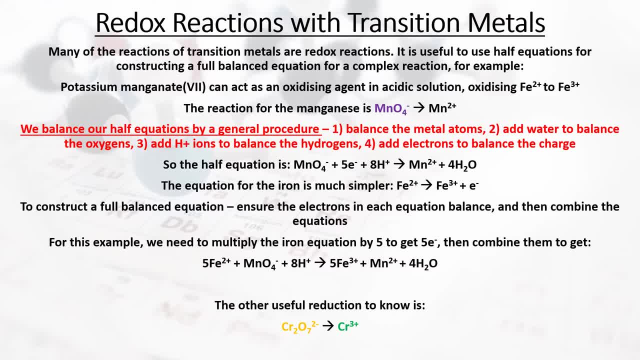 For the ion equation. we have one electron. So we need to multiply our ion equation by five to get five electrons. Once we've done that, we're going to do the next step. We're going to do the next step. Once we multiply that by five, we can simply add the two equations together. so you write. 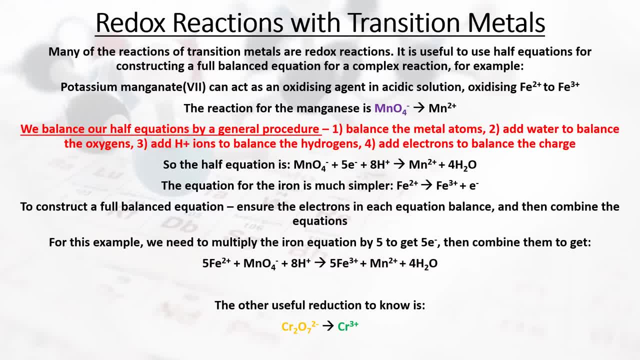 everything that's a reactant on the reactant side, everything that's a product on the product side, And by combining it you end up with five Fe2 plus plus MnO4, minus our manganate ion, plus 8H, plus going to five lots of Fe3 plus plus Mn2 plus plus 4H2O. 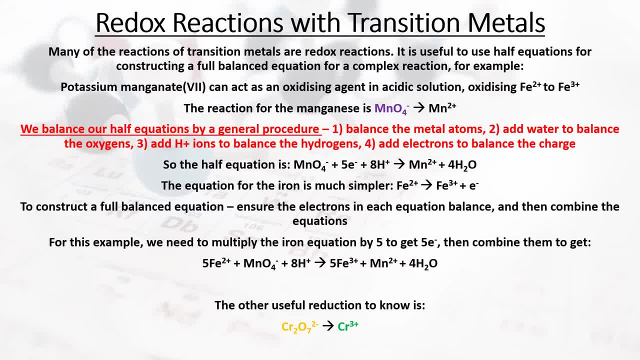 So we've oxidized our ion Fe2 plus to Fe3 plus And we've reduced our manganese. Our manganese is essentially going from the manganate 7 down to the manganese 2 plus ion. Now there are lots of different ones to know for these. 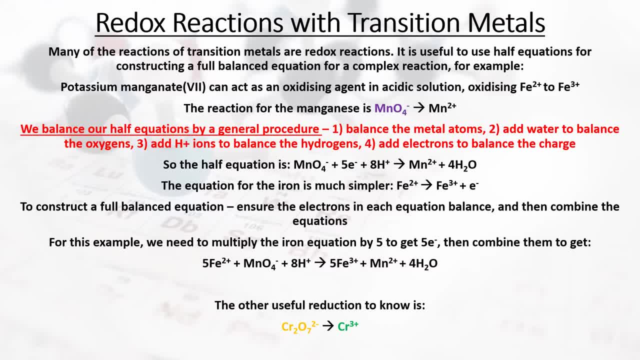 Lots of different examples they could give you of various atoms being oxidized and reduced. The other really useful one to know is actually our reduction of the dichromate anion Cr2O7, 2 minus sort of orange-colored ion being reduced to the chromium 3 plus ion. 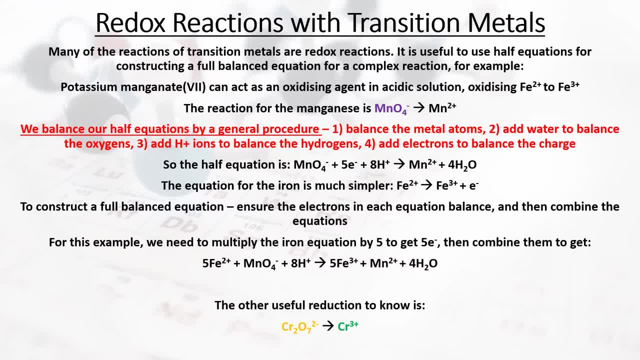 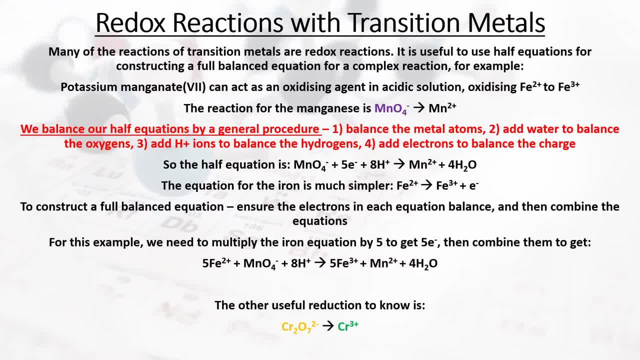 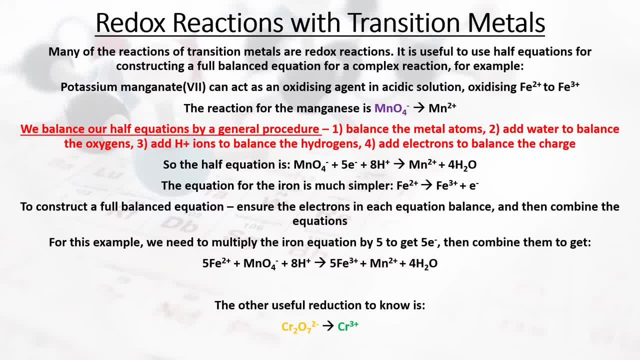 primary alcohols up to aldehydes or carboxylic acids or secondary alcohols up to ketones. This is the oxidizing agent we use normally acidified potassium dichromate, so K2Cr2O7 2 minus acidified with sulfuric acid. dilute sulfuric acid. 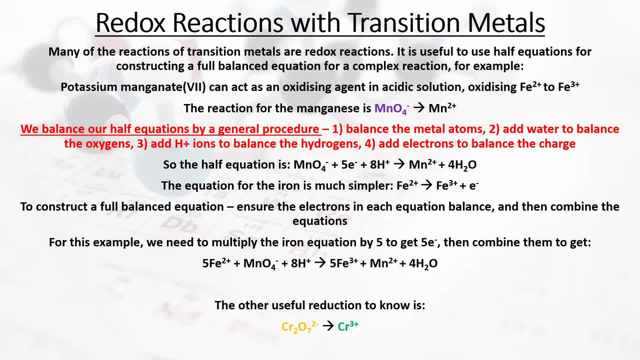 And we talk about in those reactions, that the key observation that we saw- if we've oxidized our alcohol, The key observation is that we have this color change from orange to green and that's because we've had our alcohol oxidized up to some sort of carbonyl compound and we've 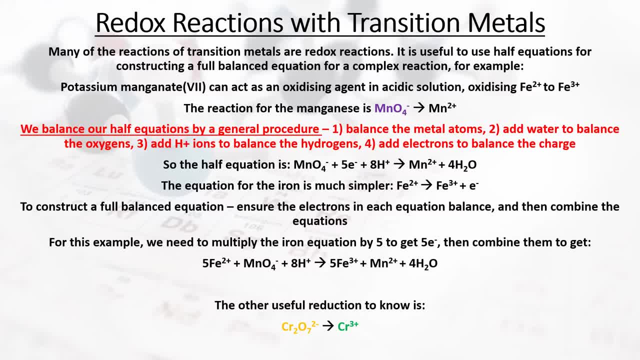 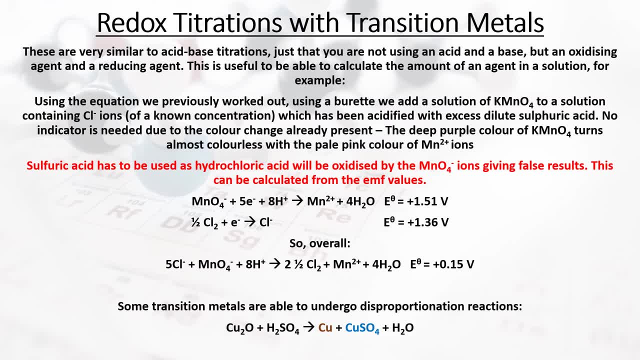 had this chromium reduced from chromium 6 down to chromium 3.. Now the next thing to talk about is doing redox titrations. So doing redox titrations with transition metals it's very similar to doing an acid base titration. 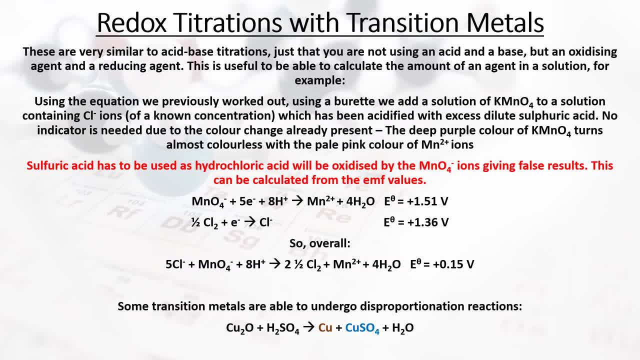 So if we think back to an acid base titration, we normally have maybe an acid of an unknown concentration. We take a base of a known concentration, react a specific volume of that base with a specific volume of the acid. We normally have an indicator present as well where we see this color change that tells 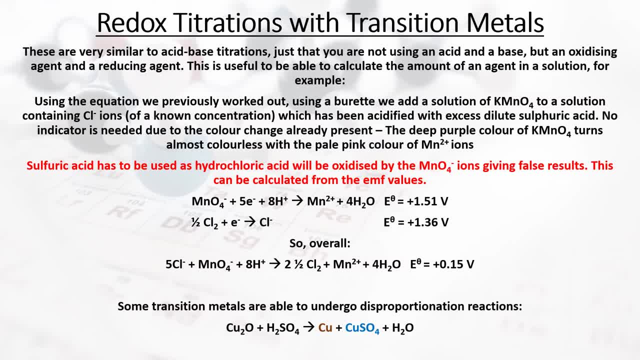 us that we've reached what we call our equivalence point or our neutralization point, And then, from using our mathematical skills, that we know that the moles equals the concentration times the volume, and we use the mole ratios that are present in our balanced chemical 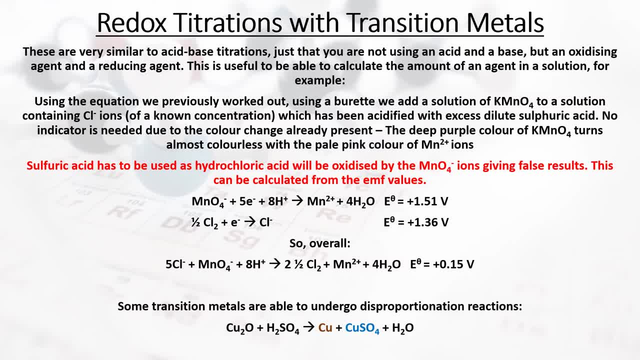 equation. We can work out what the concentration is. We can work out what the concentration is. We can work out what the concentration of this acid was. Now in a redox titration. we're not using an acid in a base, but an oxidizing agent. 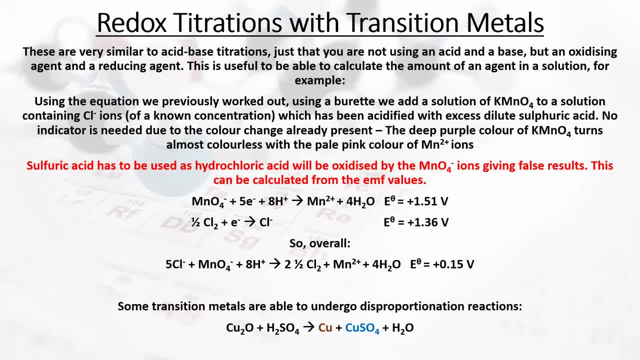 and a reducing agent, So something that gets oxidized, something that gets reduced, And this is useful to be able to calculate the amount of a particular agent in solution. So an example is that we can use the equation we've just previously worked out, that half. 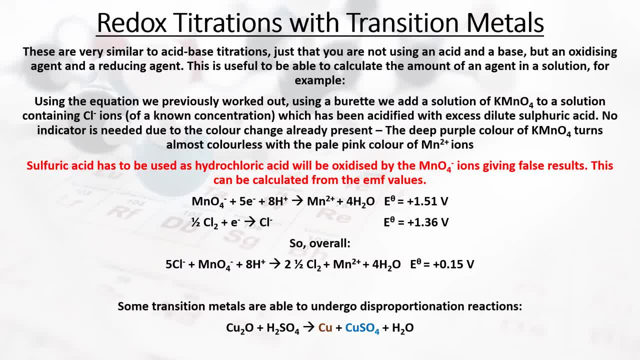 equation for the manganate ions being reduced to the Mn2 plus manganese ions, and we can see that we've reduced the madder, And the answer for that is that we've reduced the madder with a greater concentration, And so we can use that and we get the solution of our potassium manganate to a solution that. 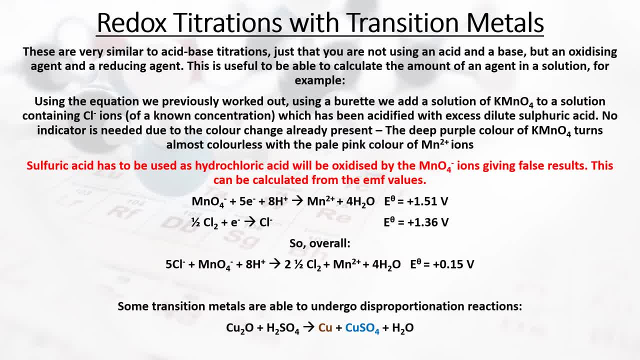 contains, for example, chloride anions. Now, we know the concentration of our chloride anions, but we don't know the concentration of our potassium manganate solution. We've also acidified this with excess dilute sulfuric acid, And actually there's no indicator required here. 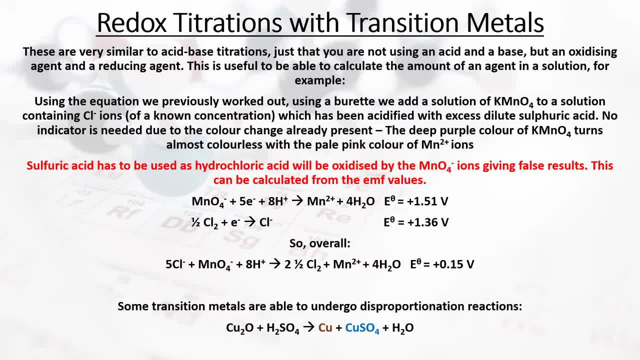 And typically for a lot of redox titrations we don't require indicators because we're we have a natural colour change already present. One of the key things here with using transition metals is, of course, that we have variable oxidation states, but also ions that typically 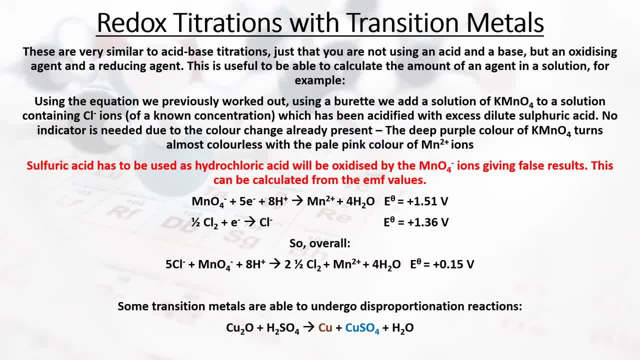 are coloured and typically different oxidation states have different colours, And so in the case of this one, we have our deep purple colour of our manganate anions, that Mn in the 7 plus oxidation state, turning to the almost colourless, very pale pink colour of the manganese 2 plus ions. So we 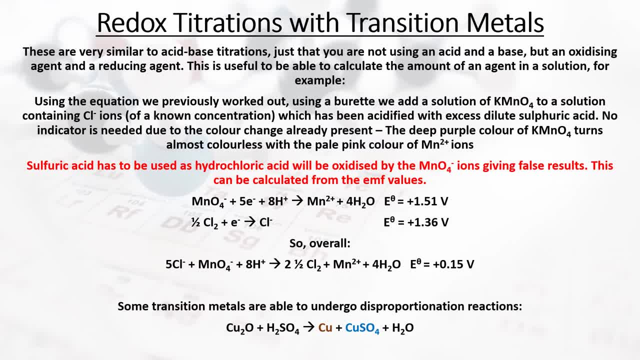 have a natural colour change anyway, so we don't need to put an indicator in, And so, in terms of the acid here we have to use sulfuric acid rather than hydrochloric acid. The reason for this is because, actually, the hydrochloric acid will be oxidised by the manganate ions and this will give 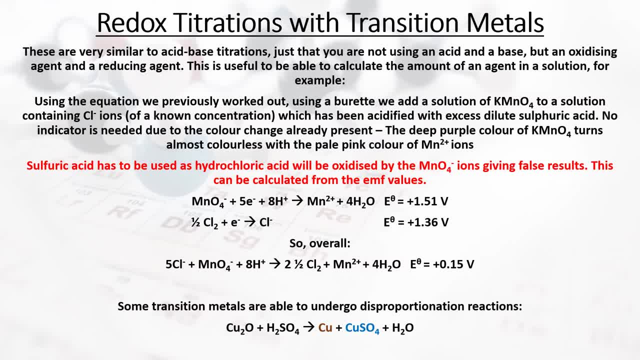 false results by introducing our intentionally introducing chlorine into our system. Now this can be calculated by looking at the emf values of the half equations for the hydrochloric acid and for these manganate ions here. I'm not going to go through this here, but 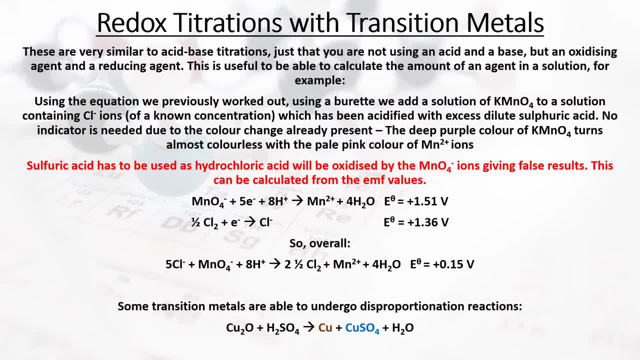 you'd be able to see that essentially, it would oxidise up the hydrochloric acid, which is not what we want, give a false positive. So we have to use sulfuric acid instead, which isn't going to be oxidised by our manganate ions, And so we have our two half equations here, we have our manganate. 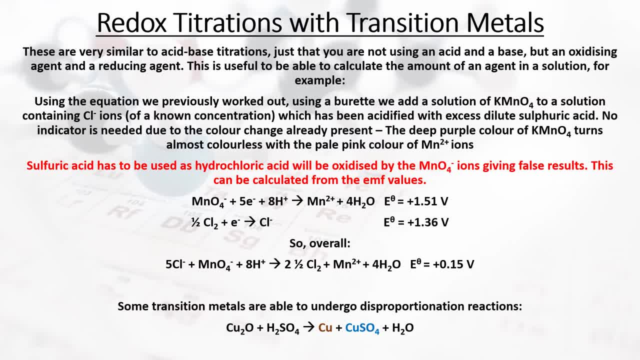 half equation that we've worked out on the previous slide. This has a potential here, a plus 1.51 volts. We then have this chlorine half equation. again, these are both written as electrochemical reductions. We have a half cell value for this being 1.36 volts positive 1.36. 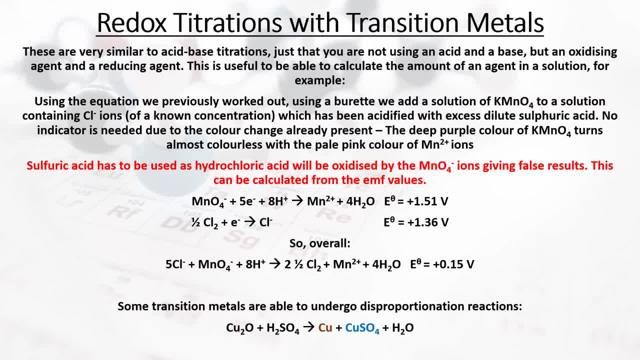 volts, And so remember that the more negative one is going to be the one that releases the electrons, it's going to be the one that is oxidised, the better reducing agent, while the more positive one is the one that is going to be reduced. 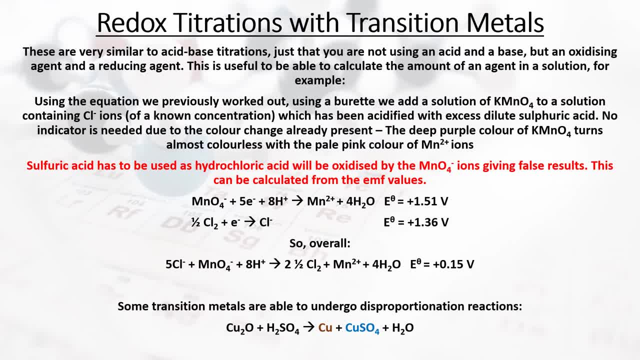 And so in this case, this works very well. we have our manganate equation being the more positive one being reduced. that's what we want. we want to reduce our MnO4 minus down to Mn2 plus, And therefore we're going to actually oxidise our chlorine equation. So we're going to have 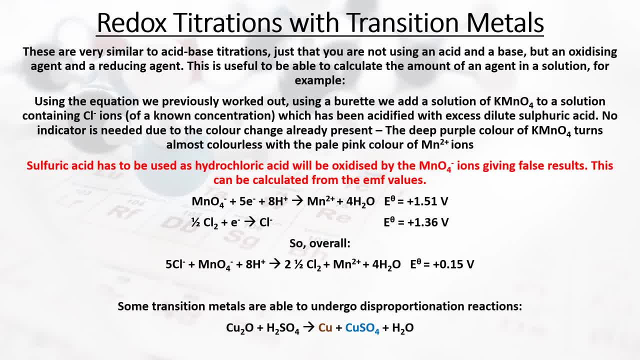 to flip our equation around. so we're going to have chloride anions releasing electrons and producing Cl2.. So we're going to flip that equation around: our manganate one we keep written as a reduction And then remember to create the overall equation we need to make. 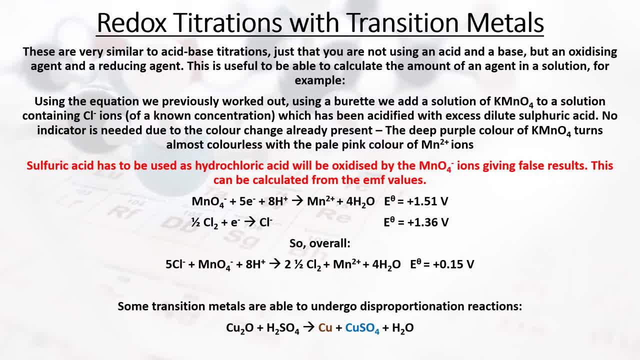 sure that our electrons balance so they can cancel out. So we have to multiply this chlorine equation by five to get five electrons that will cancel. with the five electrons in the top equation We then add together all of the reactants on the reactant side: add: 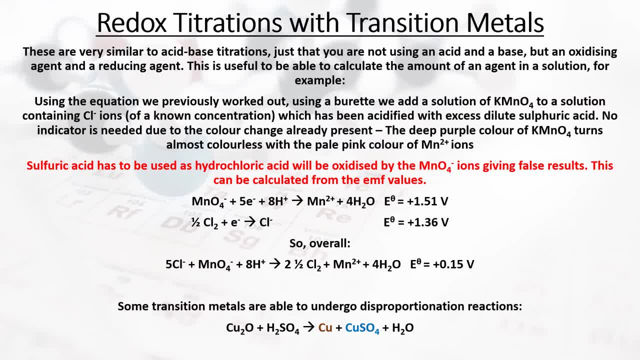 together all the products on the product side, cancel out the five electrons on both sides and our overall equation comes out to be five Cl minus plus our manganate ion plus 8H, plus going to two and a half chlorines plus Mn2 plus plus 4H2O, And again we can. we can work out our standard cell. 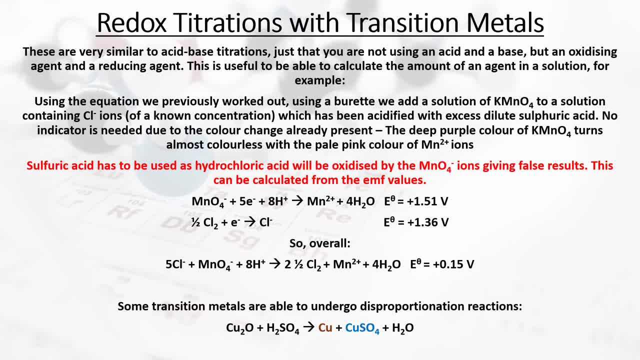 potential here. In this case it ends up coming out to be plus 0.15 volts. Now I've not drawn out, obviously, the actual sort of uh. when we calculated E cell values in the electrochemical videos, we looked at drawing them out in a specific orientation: that the thing that was reduced goes on the right. 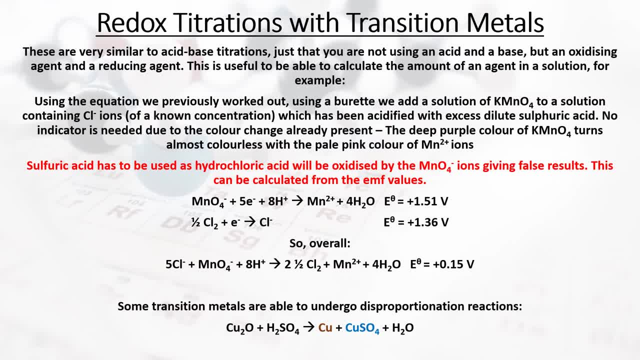 the thing that was oxidised goes on the left. Remember that when we work out our E cell values we do the right minus the left, and the right is what's reduced. So our manganate equation minus the chlorine equation gives you an E cell value of plus negative, plus 0.15.. 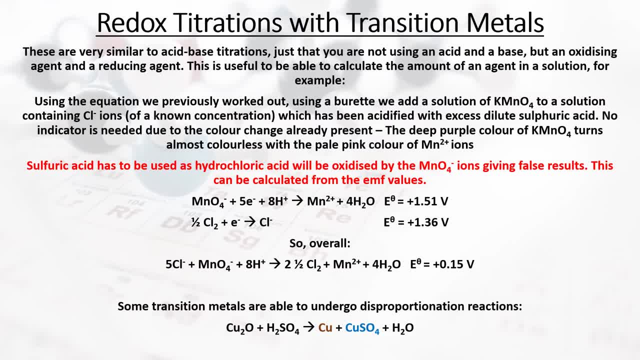 1.15 volts, a feasible reaction. Now some transition metals are able to undergo disproportionation reactions. Now, if you remember, disproportionation reactions are reactions in which one species becomes both oxidised and reduced, So it's not like in these examples. 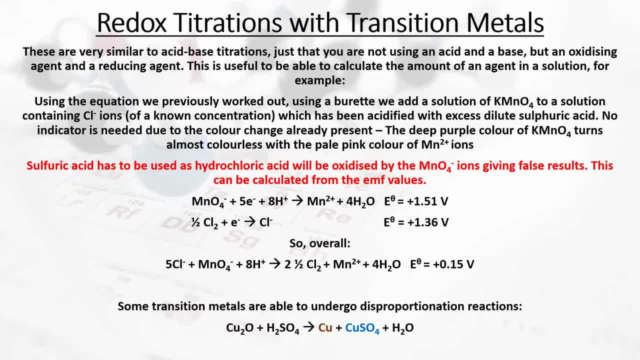 that we've had above here, where, for example, the manganate iron gets reduced and chloride gets oxidised. That's two separate species, one of them being oxidised, one being reduced. We actually have a particular element both being oxidised and reduced in the same reaction. 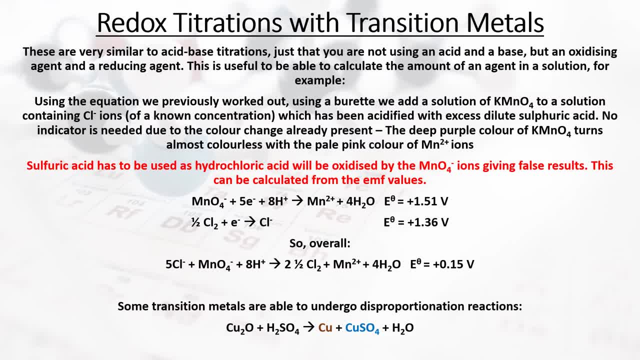 And so our example here is this: copper oxide. copper in the Cu2O Oxygen is normally minus two, and so that means that our copper here must be in the plus one oxidation state. We react that with sulphuric acid and we actually end up producing copper, copper sulphate and 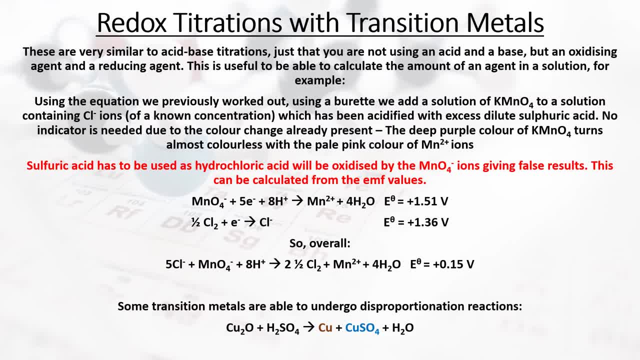 H2O. Now copper metal is kind of sort of brown Copper sulphate, of course, is probably known as a blue solution. And then we have water as well, And if you work out the oxidation states of the coppers, we've gone from plus one on the reactant side. Copper metal just being on its own has an 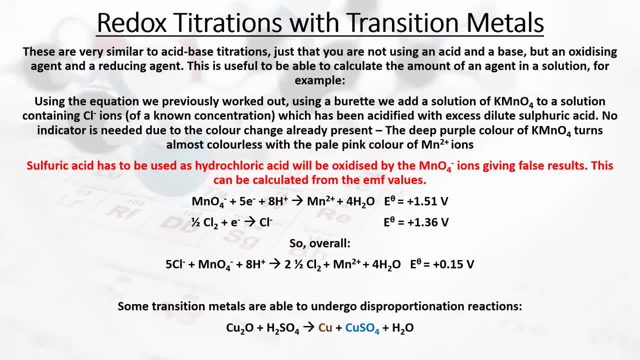 oxidation state of zero. So we've gone from plus one to zero, and so therefore we've gained, an electron must have been reduced, And then we have our copper in the plus one oxidation state going to copper in the plus two oxidation state in copper sulphate. So plus one to plus. 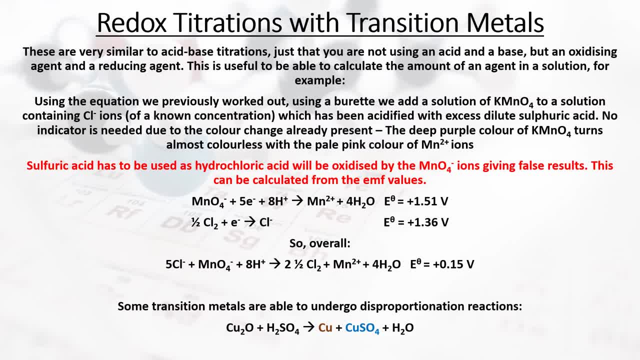 two, it must have lost electrons and therefore it's been oxidised. But the key thing is that there's an oxidation state of zero plus one to plus two, so it's been both oxidised and reduced. It's a disproportionation reaction. 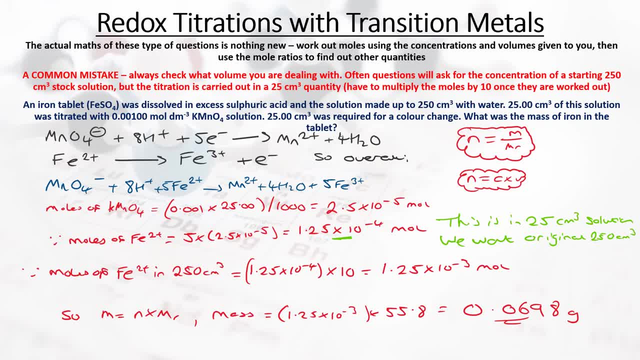 So now we can actually start to think about doing our redox titrations, actually doing some maths on these, the actual questions. So the actual maths of these questions is typically nothing new than what you've seen throughout your A level. If you go back to 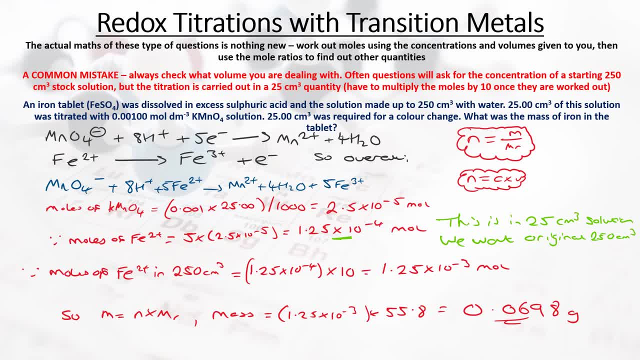 doing acid based titrations that you probably did in the first year of A level. the maths isn't really any different. We need to work out the molecules that are present in the moles using the concentrations and the volumes that we are given, and the key. 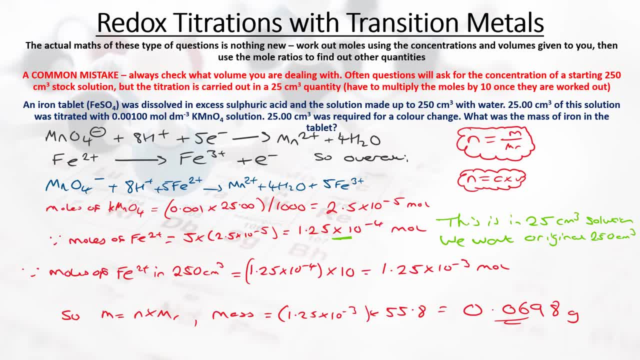 thing is that we need to use the mole ratios in the question to be able to then work out the other quantities. Now a really common mistake with these types of questions is to always triple check what volume you are dealing with. Often questions will be worded in the way that they will take you through how these 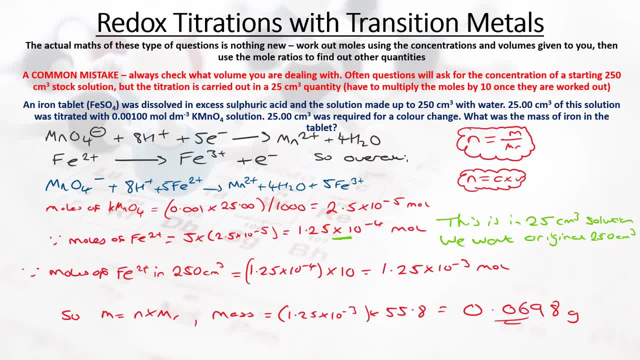 redox titrations work and they will ask you for the concentration of a starting 250 centimetre cubed stock solution, for example, But typically the titration is carried out using a 25 centimetre cubed portion of that stock solution. So you've created up your stock solution. you've then taken a small 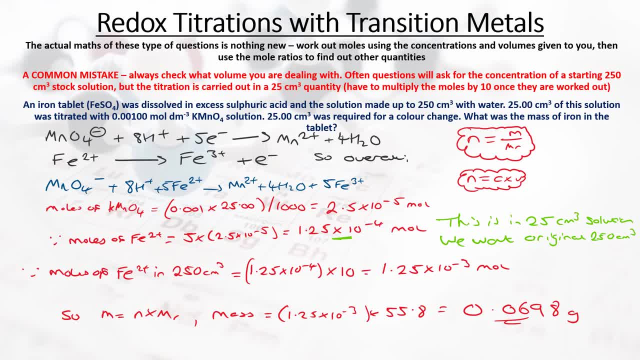 quantity- 25 centimetres cubed out of that to do the titration with- and so the key thing to remember is always remembering what is the volume that I'm actually dealing with, Typically when you work out the moles in the titrations. 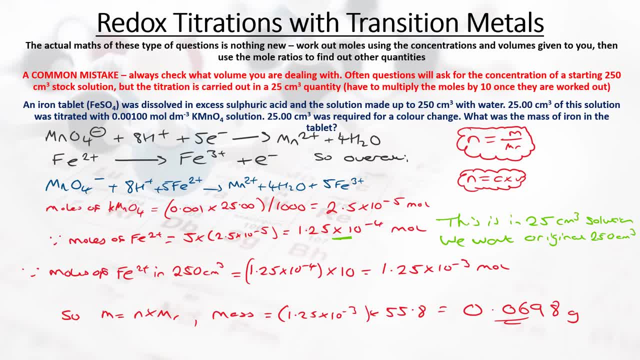 you're dealing with the smaller quantity that you've used in the titration and then the majority of the time you're dealing with the moles in the titration. but if the question asks you for this, for the concentration of starting stock solution, you have to remember to multiply the moles by 10 once you've. 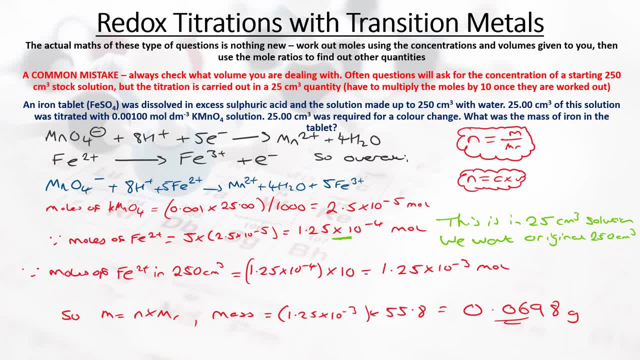 worked them out because the starting solution had 10 times the amount of the amount that you used in the titration. So an example might be an iron tablet, which is mainly iron sulfate. FES-04, was dissolved in excess sulphuric acid and 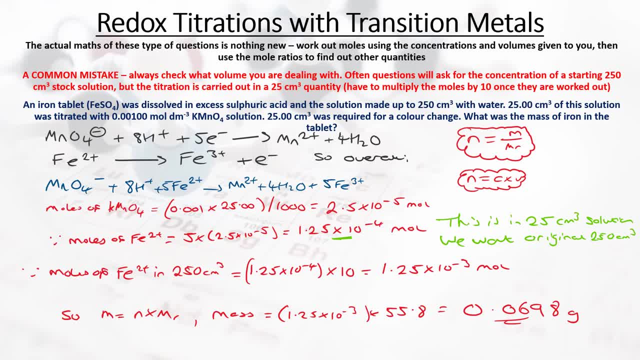 the solution made up to 250 centimetres cubed with water, So that's creating a stock solution, centimeters of that solution. we've taken 25 centimeters cubed of that stock solution and that was what was titrated, with a 0.001 mole per decimetre cubed potassium manganate solution. 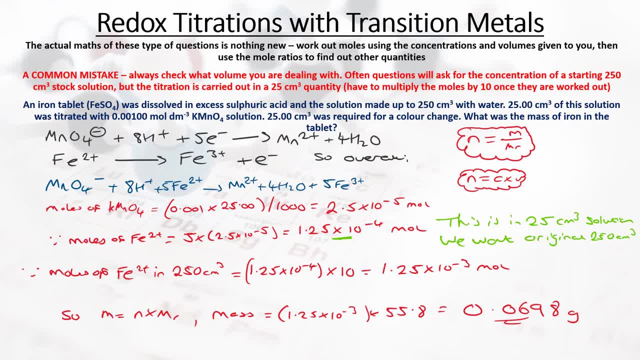 and we're told that exactly 25 centimeters cubed was required for a colour change. What was the mass of the iron in the tablet? So the way that we need to go about this is using the skills that we've just been using all the video. So we take our half equations and typically I think this: 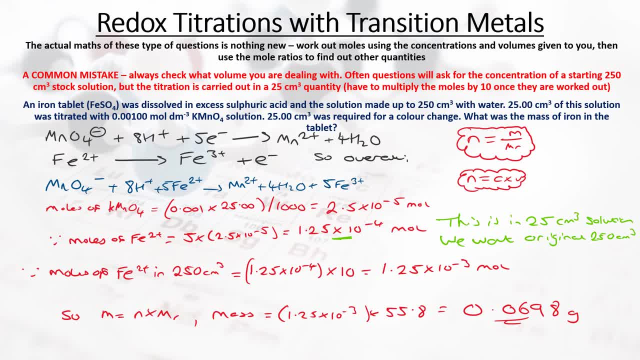 manganate equation is one that you need to remember. so it's MnO4 minus, always going down to Mn2 plus. The iron equation is what we saw earlier on. they probably give you that in the questions: Fe2 plus going to Fe3 plus. So we do what we've done in the previous few slides. we 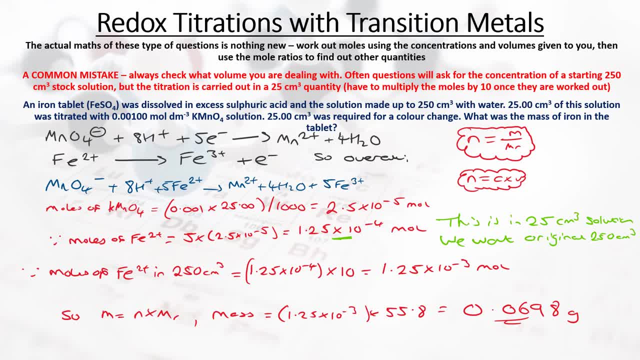 balance our half equations. I'm not going to go back through it again. balance it up with waters and hydrogen ions and electrons to make sure that all the atoms and charges balance. We end up with these two half equations to combine them into the full equation. remember we have to get our 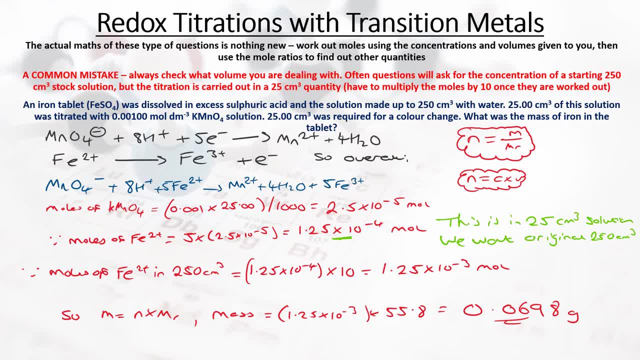 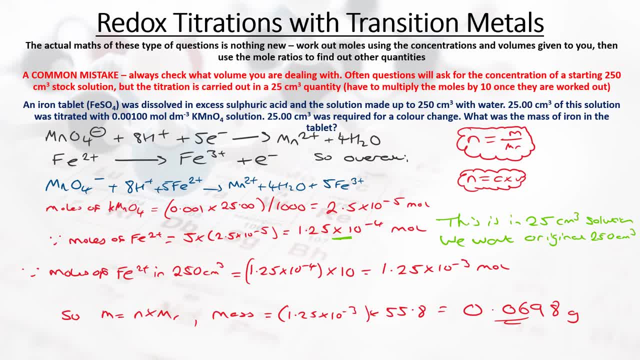 the products on the product side, cancel out your electrons on both sides and your actual overall equation here comes to be our manganate ion plus Fe2 plus, going to our manganese ion, Mn2 plus 4 H2O and 5 lots of Fe3 plus. So really the two equations that we really need to use here. 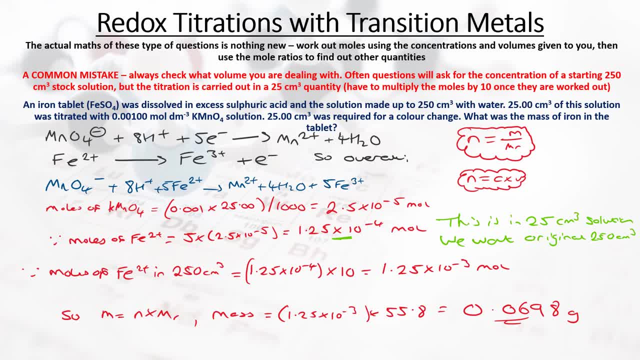 are our mole equations. remember there's two forms of the mole equation. there's the mole equation for solutions, which is concentration times volume. remember that if we're dealing with that, we have to always think about our units. concentrations are in moles per decimetre cubed. volumes are 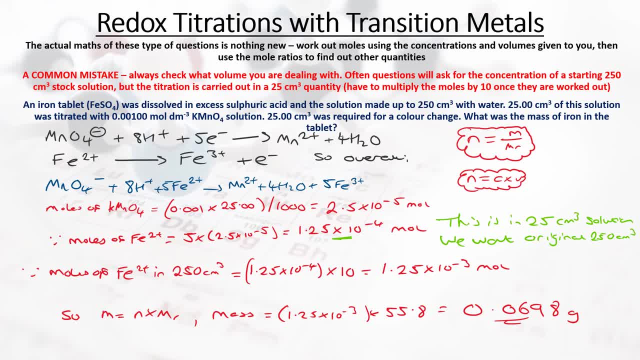 typically given in centimetres cubed. so we have to convert our centimetres cubed volume into decimetres cubed by dividing by a thousand, and the other mole equation is moles is the mass divided by the molecular mass. So if we're dealing with questions like this and, as I always recommend, with mathematical questions, 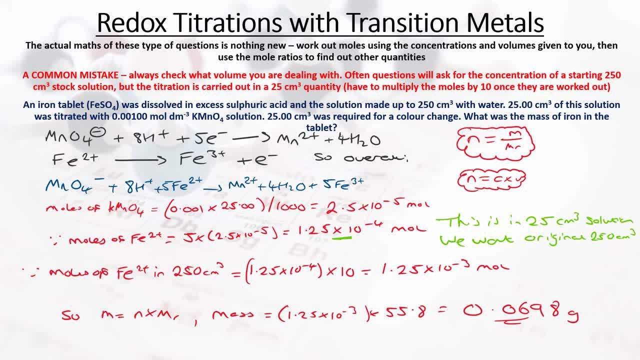 even if you're not sure how to start a question, simply use the data that you've been given in the question, so you're told a volume and a concentration for the potassium manganate. if you have a volume and a concentration, you can work out the moles, even if we're not sure what we're going to do. 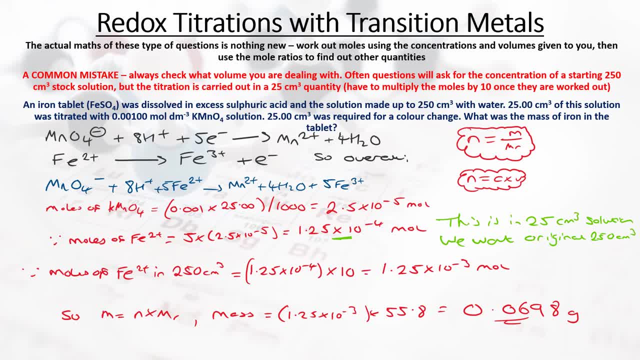 with it. work out the moles- you'll get a mark for doing that- and so our moles of the potassium manganate. we're given a concentration and the volumes we use the N equals C times V, remembering to divide by a thousand to convert our centimetres cubed volume into a thousand. and that's what we're. 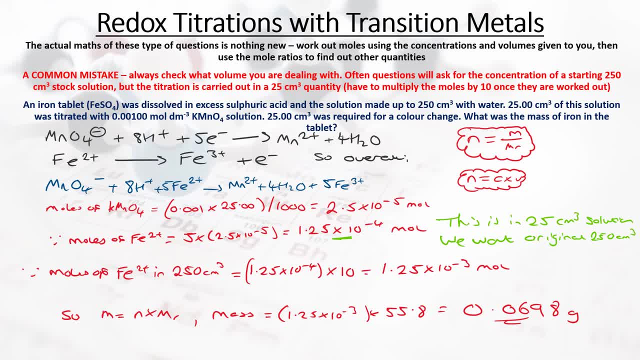 going to do? we're going to convert that into a decimetres cubed volume. so we do 0.001 times the 25 divided by a thousand, and this gives us 2.5 times 10 to the minus 5 moles. so that's. 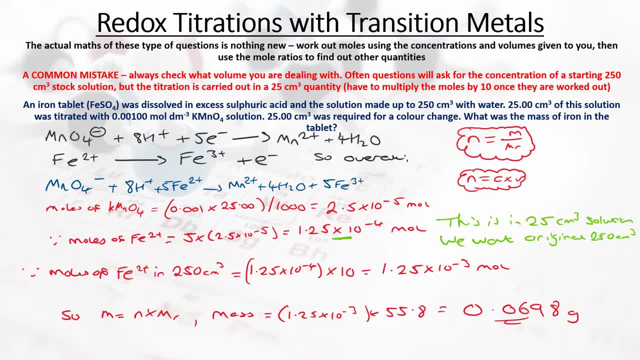 our moles of potassium manganate. what we want, though, is to be working out the maths for the iron. we want the iron tablet maths, essentially the mass of the iron in the tablet, so we have to then think: this is where it's really important to use our mole ratios. what's the mole ratio of? 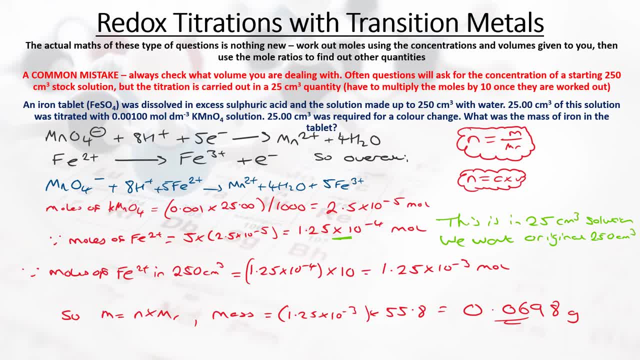 the manganate compared to the iron, two plus, and you can see from our overall balanced equation that we have one mole of manganate, MnO4 minus, reacting with five moles of Fe2 plus. so to work out the moles of Fe2 plus we simply multiply the moles from the 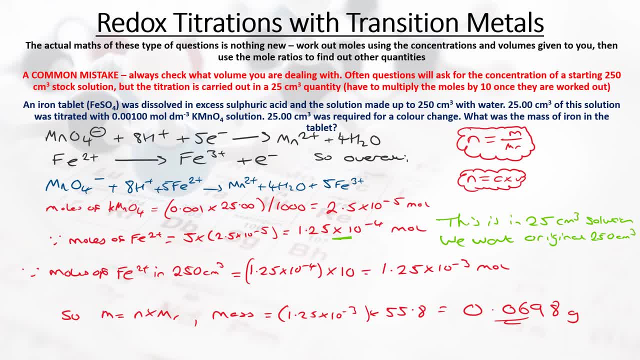 previous line of working. by five, that gives us 1.25 times 10 to the minus four moles. now this is the point where it's really important to remember what concentration, what volumes are you're dealing with and typically, sometimes- I haven't drawn it on here, but sometimes in. 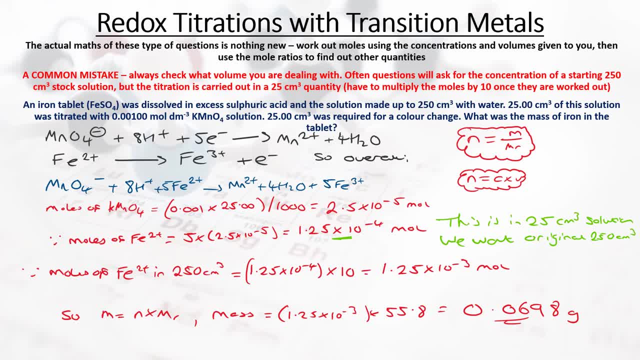 questions like this. I'll actually draw a little diagram out to remind me the steps we've made. okay, we've taken that 250 centimeter cube stock solution for our from our iron tablets and then we've taken a small portion of that 25 centimeters, cubed a tenth of it out to do the titration. so 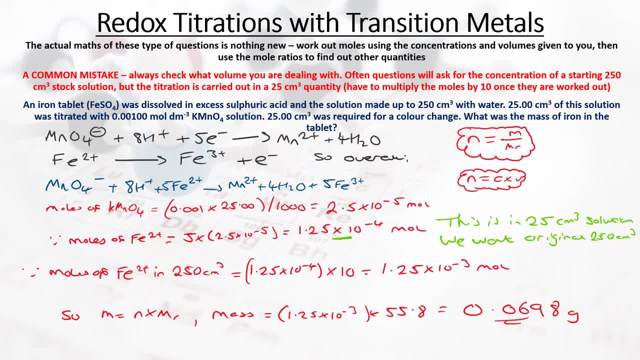 this moles of Fe2 plus that we've worked out is actually for the, the 25 centimeter cubed solution. Our moles have been worked out, worked out from the titration data. however, the question asked us for what was the mass of the iron in the tablet? That tablet was dissolved in the 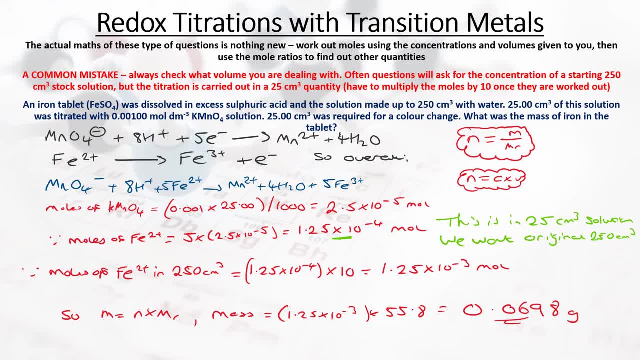 250 centimetres cubed. So we need to multiply the difference. the 25 centimetres cubed going into 250 is 10, so there's 10- lots of that in our 250 centimetres cubed solution. so 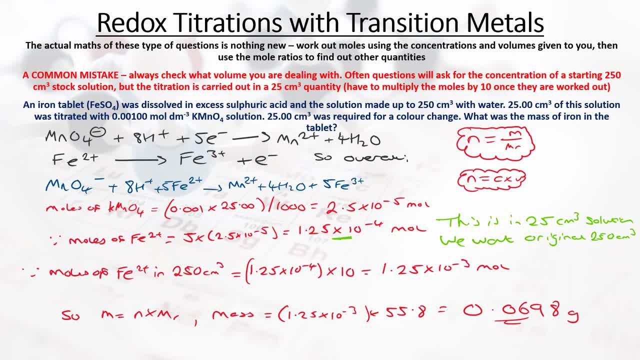 we multiply our answer by 10, and so the moles of the Fe2 plus in the original 250 would have been 1.25 times 10, to the minus 3 moles, And then once we have the moles of our iron, 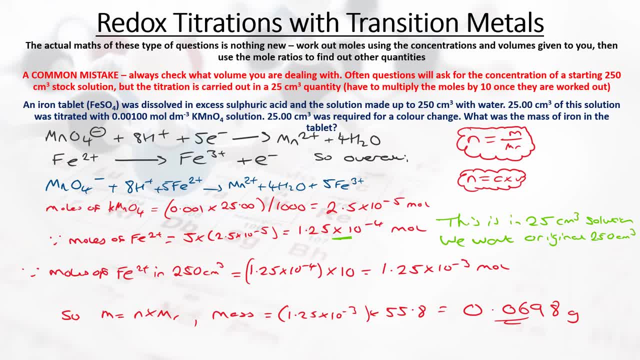 2 plus, we can then work out the mass of the iron, and so, therefore, we just need to use our moles as mass divided by Mr, rearrange it for mass. so mass is moles times Mr, and so we do the moles multiplied by the molecular mass of our. we're concerned about the iron. 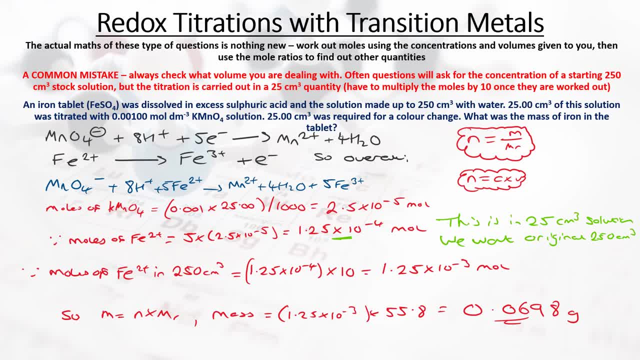 the Fe, which is 55.8, and therefore we take it. we take the 55.8 multiplied by our moles in 250 centimetres cubed and that gives us 0.0698 grams. And again, watch the significant. 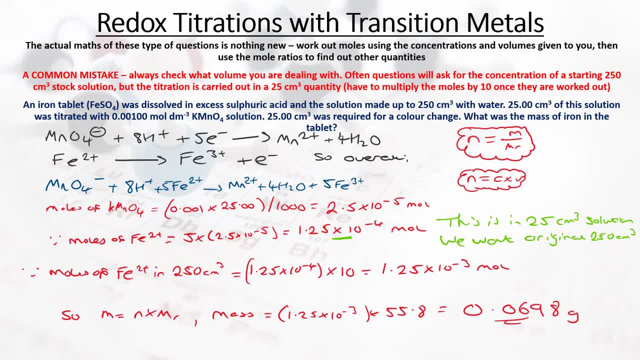 figures. we can only give our answer to the minimum, The minimum number of significant figures in the question. the 250 centimetres cubed is a three decimal, three significant figures. our 25 centimetres cubed is four significant figures technically and our 0.001, notice we have two zeros at the end of that. that's. 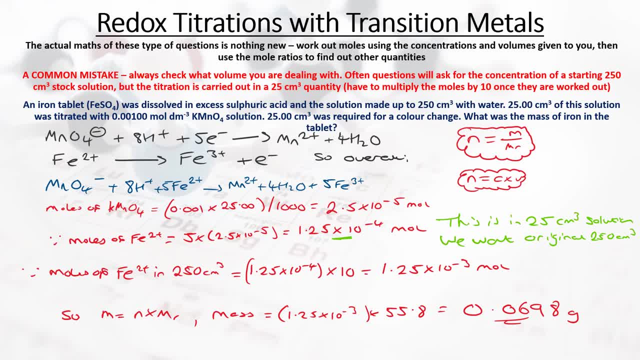 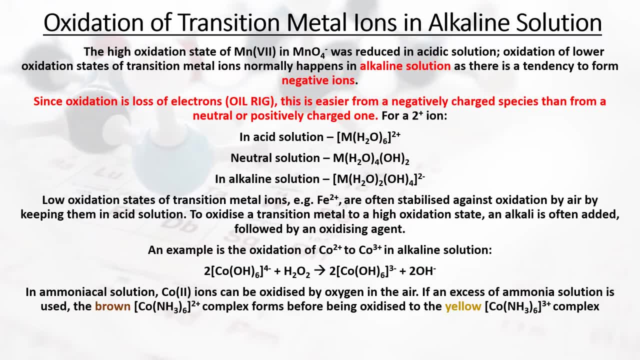 also a three significant figure number, And so therefore the minimum is three, so we give it to three significant figures: 0.0698.. And so the final thing to talk about here is our transition metal ions, actually how we oxidise our transition metal ions in alkaline solution. 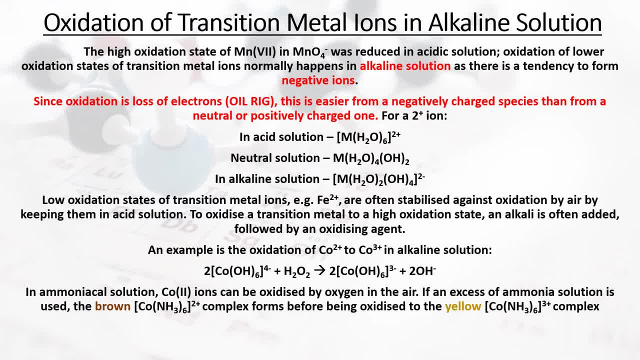 rather than acidic solution. So we saw just now that the high oxidation state of our manganate ion, our MnO4-, our manganese, here in the 7 plus oxidation state, was reduced in acidic solution. We also saw that that could happen if we had our dichromate anion, our chromium. 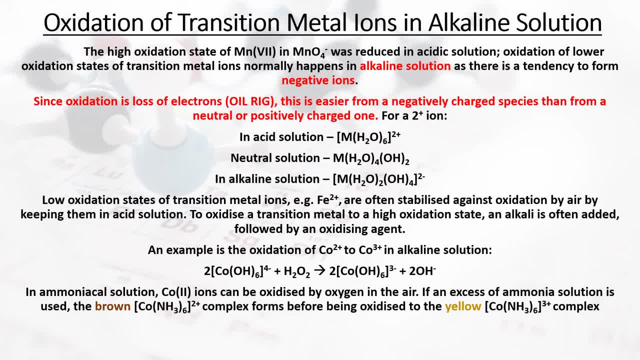 in the plus six oxidation state. again, a very high oxidation state was reduced in acidic solution. The oxidation of lower oxidation states- transition metal ions- normally happens, though, in alkaline solution, And this is because there's a tendency to form negative ions in alkaline solution. 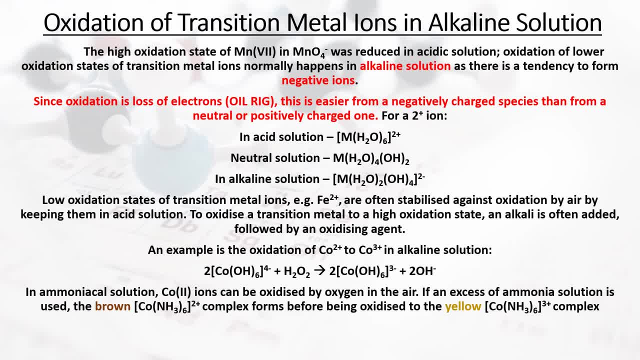 And since oxidation is the loss of electrons- remember oil rig- oxidation is loss. the loss of electrons is easier from a negatively charged species than from a neutral or a positive one. You can think of this as being: if it's already negatively charged, it's happy to. 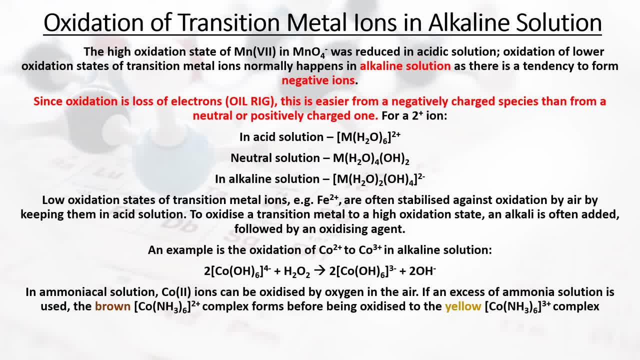 lose electrons because we have this kind of repulsion between the electrons that are in negatively charged and the actual negative charge overall on the ion, It's happy to lose the electrons essentially, And so if we take this as to kind of an overall two plus ion if we're in acidic solution, 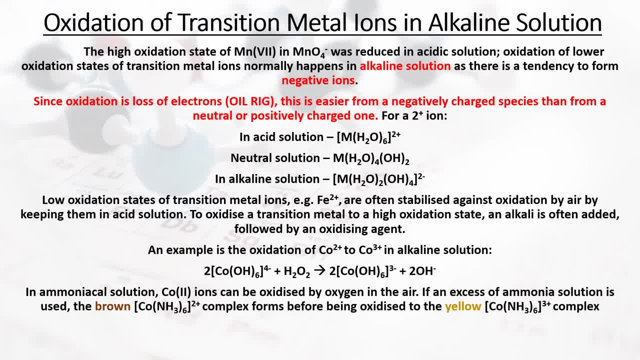 that normally exists as our hexa-aqua ion, the M H2O6, two plus ion In a neutral solution. this would be typically our precipitate of this, so our neutral metal hydroxide precipitate. So we can normally think of that as sort of being M 0H2.. 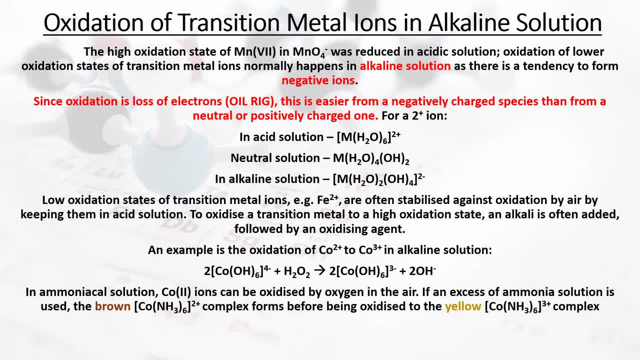 But of course, remember that we're in aqueous solutions, so we also have our water molecules there as well, so M, H2O4, OH2.. In alkaline solution we typically end up forming negative ions. In acidic solution, we normally form positive ions. Alkaline solution, though, is normally negative ions, And so therefore, 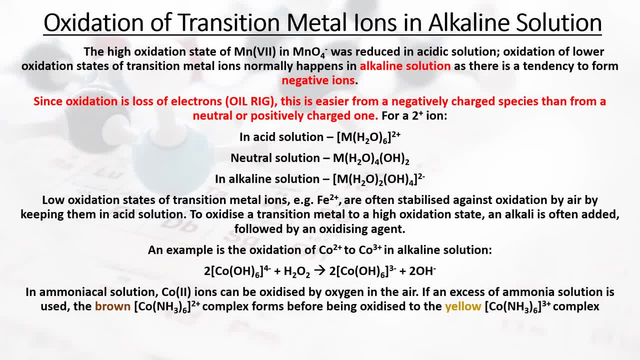 we end up forming this M, H2O2, OH4, two minus. So now we've essentially gained more of those OH minus, those alkaline OH minuses, And so the low oxidation states of transition metals, for example the Fe2 plus they're. 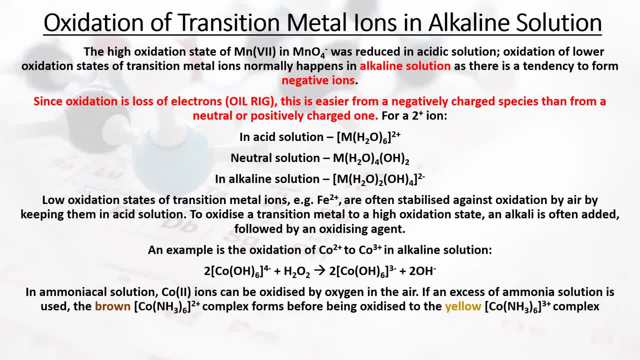 often stabilised against the oxidation by air. So if I left Fe2 plus ions just in open to air, these would be quite quickly oxidised up to the Fe3 plus ions. Now they're often prevented against this oxidation by air by keeping them in an acidic solution where it's 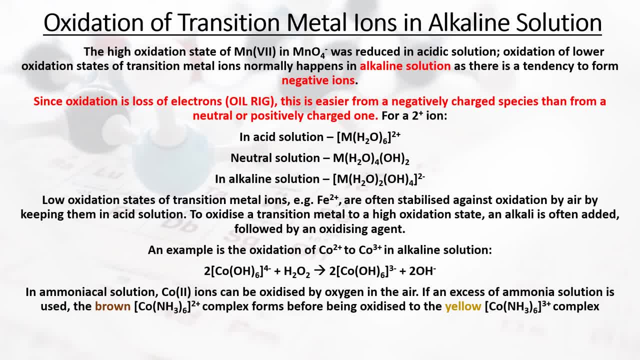 harder for these things to be oxidised. Typically we reduce things in acidic solution, we oxidise things in alkaline solution And so to oxidise a transition metal state up to the high oxidation state. so let's say we're going from our chromium 3 plus up to the chromium 6 plus in our dichromate or 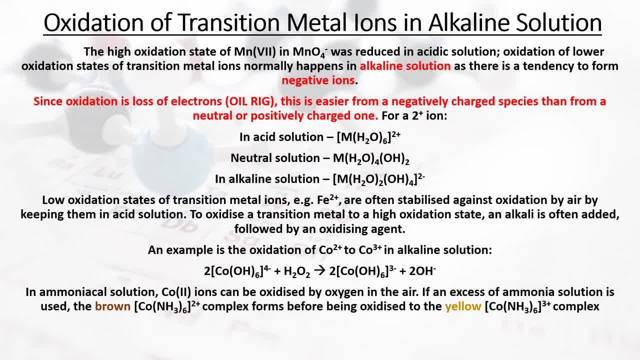 the manganate 2 plus up to the Mn7 plus. in our manganate ion often an alkali is added, followed by the oxidising agent. The alkali essentially forms our negative ion. We then have our oxidising agent, where it's easier to actually oxidise that metal because it's 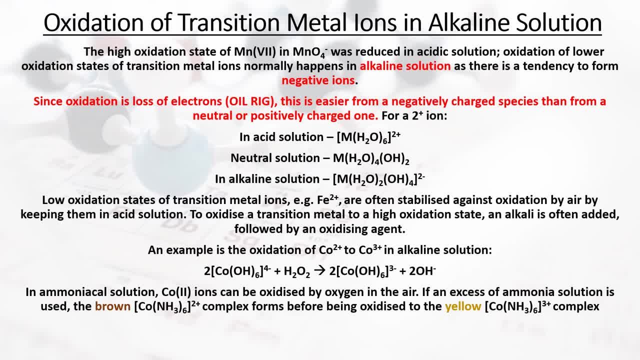 from a negative ion, And so an example is the oxidation of this cobalt 2 plus ion to the cobalt 3 plus in alkaline solution. And so you can see, here we have our cobalt with six hydroxide ligands, OH. 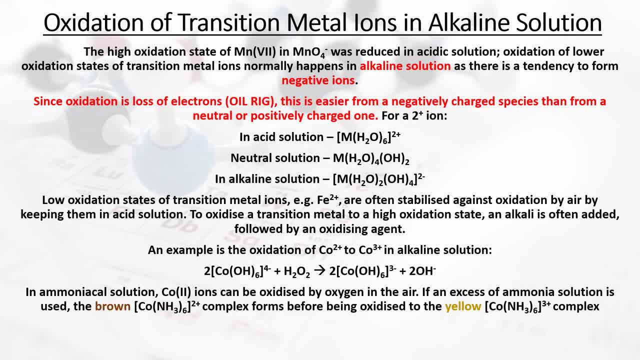 ligands, that's a four minus ion. We have our hydrogen peroxide and then this ends up oxidising. hydrogen peroxide ends up oxidising this alkaline solution of our cobalt up to the cobalt 3 plus ion. So again, you can see there that we have this same, the same ligands. 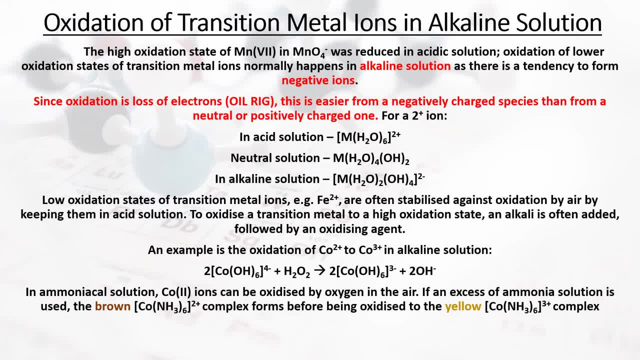 essentially six hydroxides. We've just gone from a cobalt 2 plus ion to a cobalt 3 plus ion. Now, if we're in an ammonia solution, these cobalt 2 ions can actually be oxidised by oxygen in the air, And if we use an excess of ammonia solution, then we have a ligand. 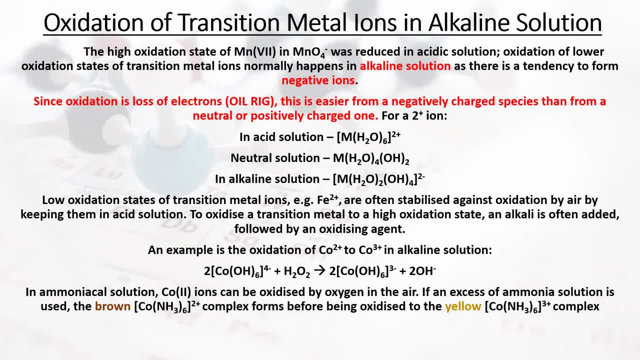 substitution reaction taking place, where we end up then producing a cobalt hexa-amine complex, cobalt NH3 6, 2 plus. These are brown, And if we have these hexamine complexes, they can be oxidised by the oxygen in air. 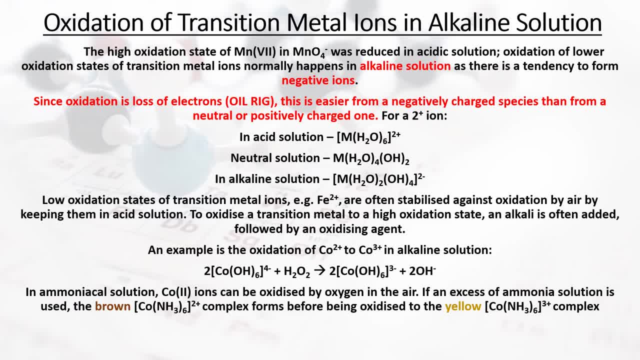 They're not protected by being in this alkaline environment. They're not protected in that way, And so they can be oxidised by air up to the cobalt 3 plus ion. So we now have our cobalt NH3 6, 3 plus ion. 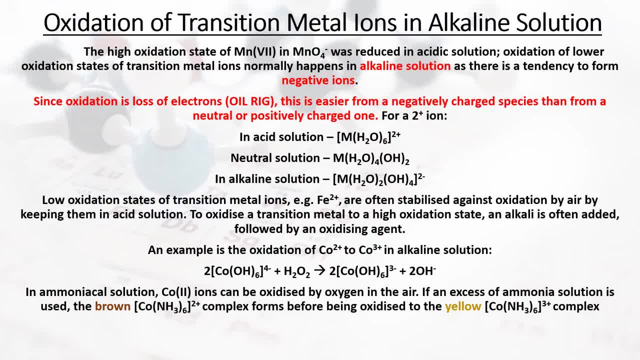 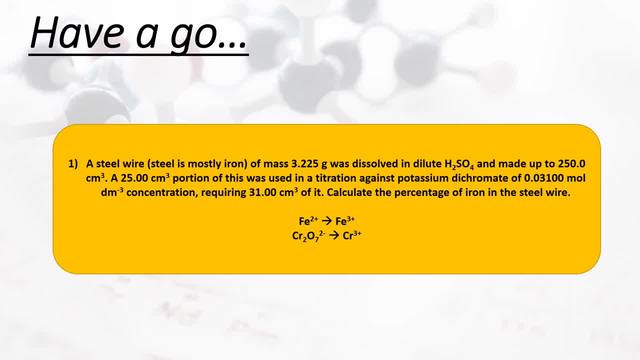 And this is a yellow colour. So time to have a go at a question. Just one question this time, but it's going to use all the skills that we've talked about in this set of videos. So it's a redox titration question: calculating the percentage of ion in a steel wire. 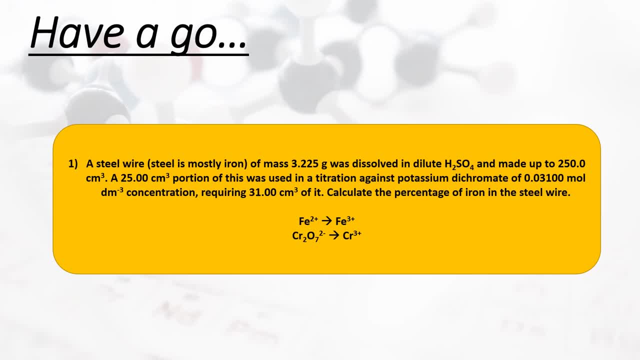 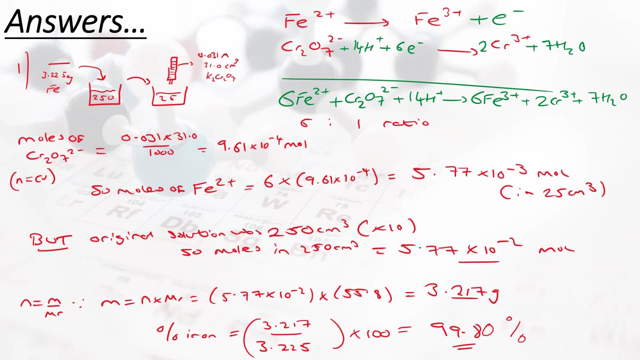 So the unbalanced half equations are given there. So have a go. pause the video and the answers will be on the next slide. So this is very similar to the example we did earlier on. Now we're using actually a chromate half equation rather than the manganate half equation. 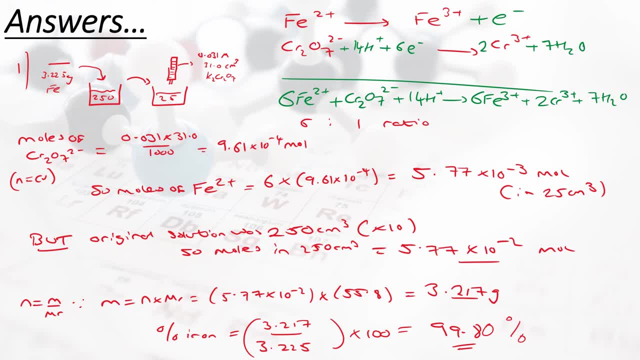 But essentially all this stuff is going to be used to calculate the percentage of ion in a steel wire. So we're going to use the two half equations that we did before apply here. So we're going to think about having our half equations, balancing these half equations by adding our waters, our hydrogen ions, our electrons in to make sure the atoms and charges balance. 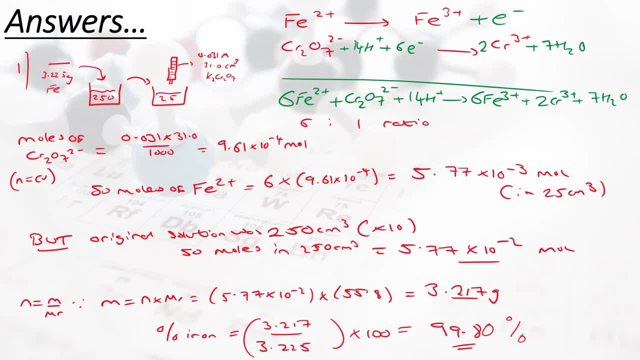 We're then going to combine our half equations, making sure the electrons balance, to get a full equation. Then we're going to use the data in the question to be able to work out moles, use the mole ratios and eventually get to our answer here that it wants the percentage of the ion in the steel wire. 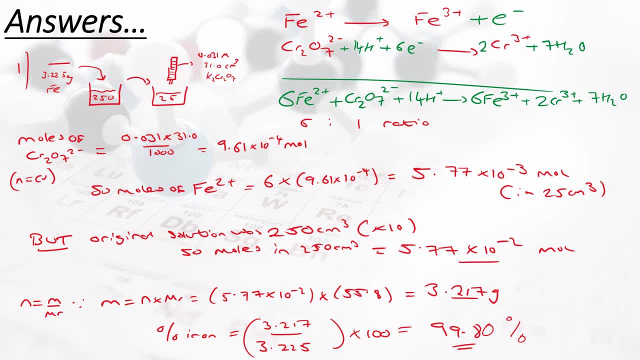 So we have our two half equations. The first one is the ion ion being oxidised from Fe2 to Fe3+. That's a very simple one to balance. We don't have to worry about waters or hydrogen ions, because there's no oxygens or hydrogens. 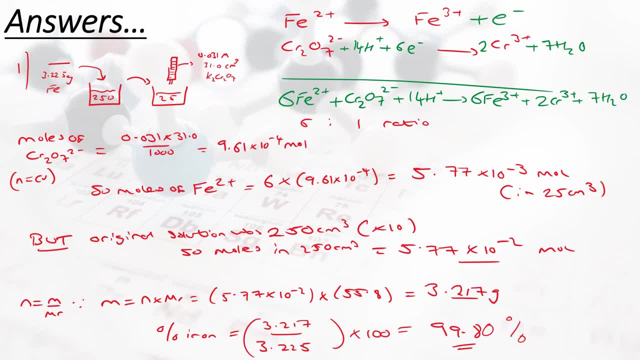 We just add in our one electron to balance the charge. The dichromate one is a bit more difficult. So we have Cr2O72-, the dichromate chromium 6+ being reduced to chromium 3+. Now, the first thing to remember from that list was to always make sure that our metal atoms balance. 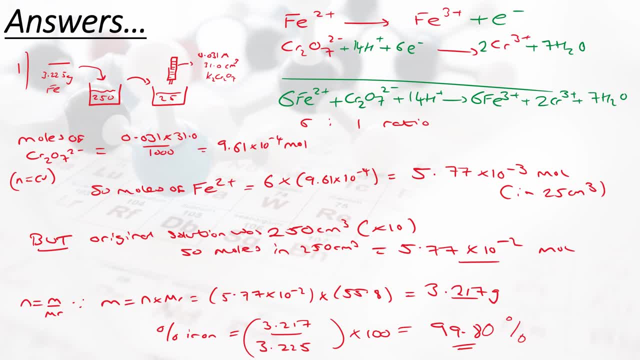 So the first thing to notice here is that we have two chromiums on the left and only one on the right, So we have to put two Cr3 on the right-hand side. We then have seven oxygens on the left-hand side, So we balance our oxygens, remember, with water. 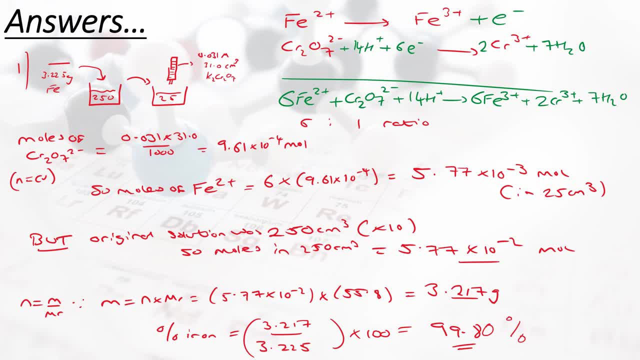 So seven H2Os on the right-hand side. We've then introduced 14 hydrogens on the right-hand side, So we have to add in 14 H+ on the left-hand side, And then, finally, we have to balance up our charge. 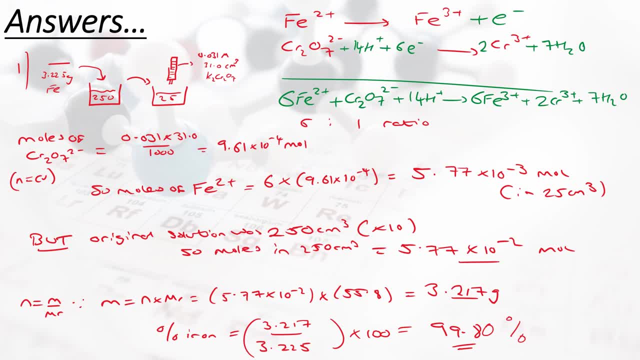 So on the right-hand side we have an overall 6-plus charge. To get an overall 6-plus charge on the left-hand side we have to add in six electrons. Then we note this: We have six electrons in the bottom equation, only one in the top. 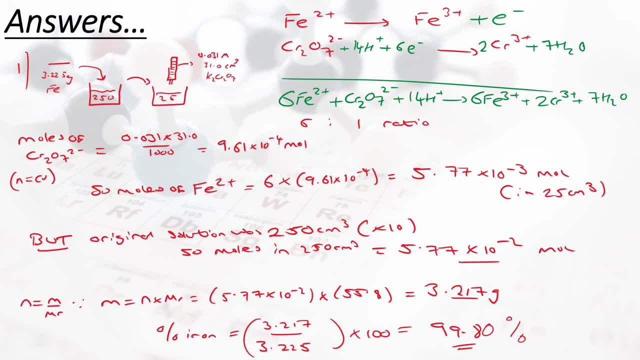 So we need to multiply our ion equation by six to get six electrons. Once we then combine these half equations, so add all of the reactants together on the reactant side, add all of the products together on the product side, we end up with our full equation. 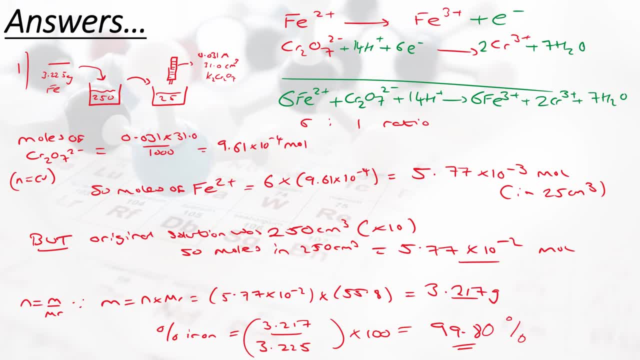 We cancel out our six electrons on both sides and our full equation is 6Fe2+ plus our dichromate anion, plus 14H+, going to 6Fe3+, two chromium 3+ ions and seven water. 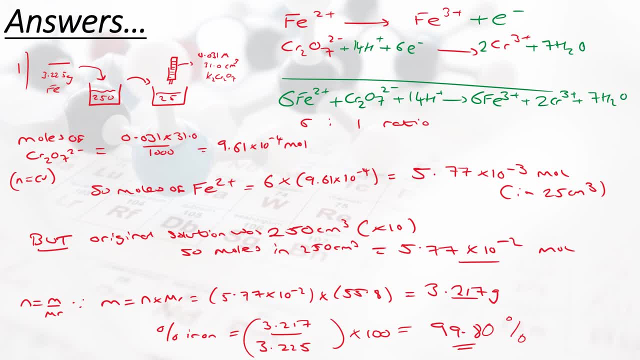 And so the key thing here is that we can see we have a six-to-one ratio of our ion to our dichromate. So in the question we were told that we had our steel wire, which steel is mostly iron mixed with a bit of carbon. 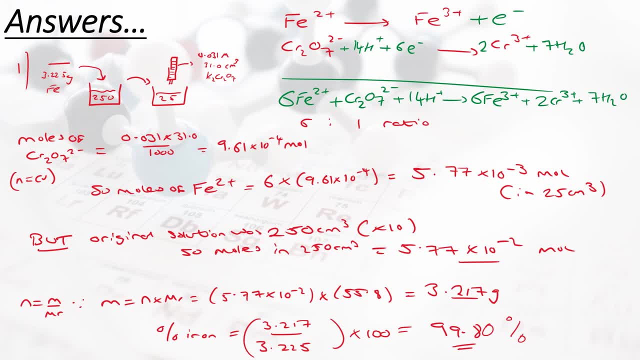 We have a mass of 3.225 grams dissolved in dilute sulfuric acid and made up to our 250 cm3 stock solution. So here we go. I'm going to draw a picture of this to help me remember what kind of volume I'm working in. 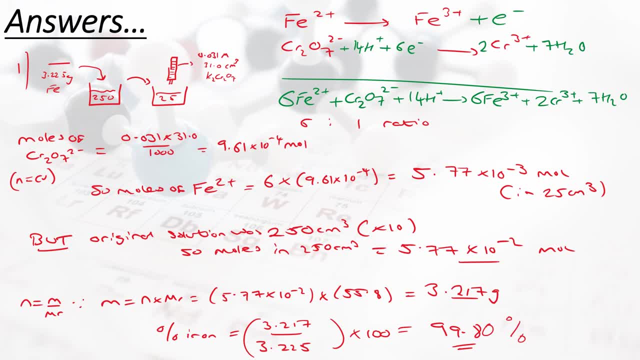 So I take my steel wire, I dissolve that up. I dissolve that up in 250 cm3 to make my stock solution. I then take a 25 cm3 portion of this and use it in my titration. So I'm going to draw essentially an arrow showing that I'm taking 25 cm3 out of that. 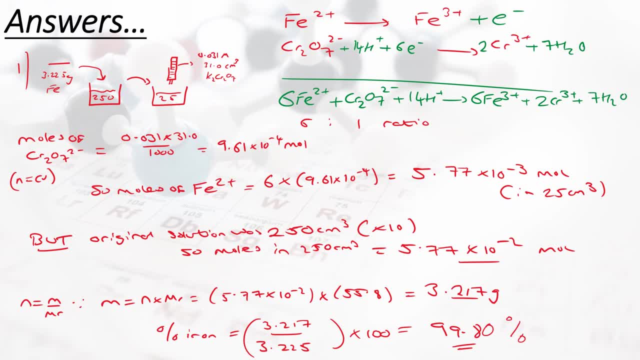 And then I draw my sort of little very rubbish drawing there of a burette to indicate that I'm doing the titration with that 25 cm3. And we were told that it required 31 cm3 of a 0.031 mol per decimetre cubed. 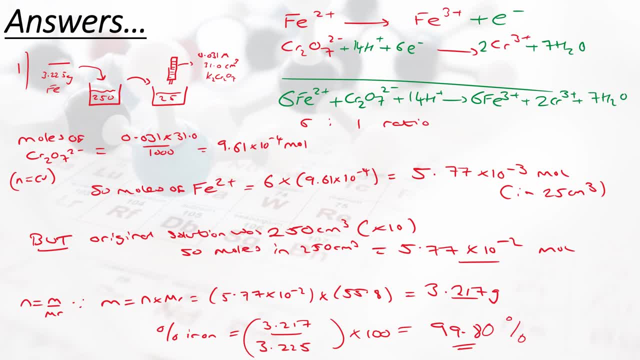 So that's the concentration solution of our potassium dichromate. So again, even if we're not sure what to do, use the data the question gives us. We've given a concentration and a volume for the potassium dichromate so we can work out the moles. 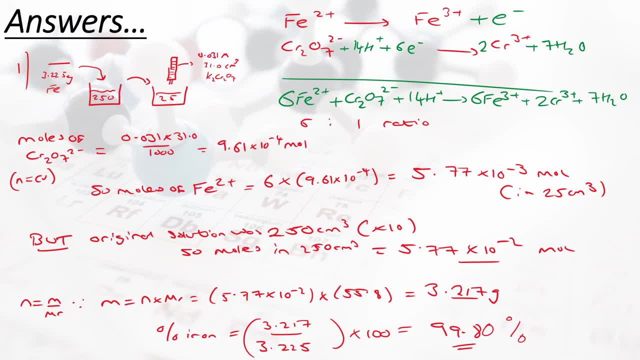 That's by doing our moles as concentration times volume, Remembering that we have to turn our volume from centimetres cubed into decimetres cubed by dividing by a thousand. So we do put those numbers in the 0.031 multiplied by 31 divided by a thousand. 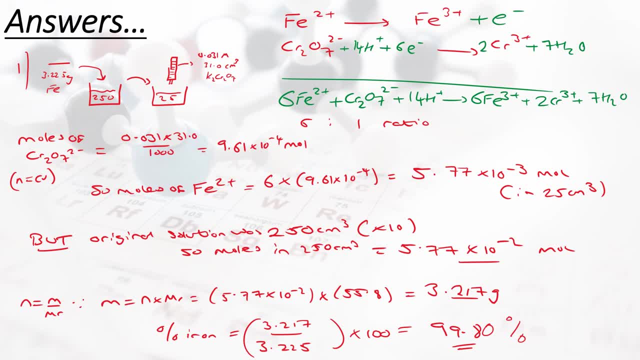 And this comes out to be 9.61 times 10 to the minus 4.. We then use our mole ratios here. So for every 1 mole of our dichromate we have 6 moles of iron, 2 plus. 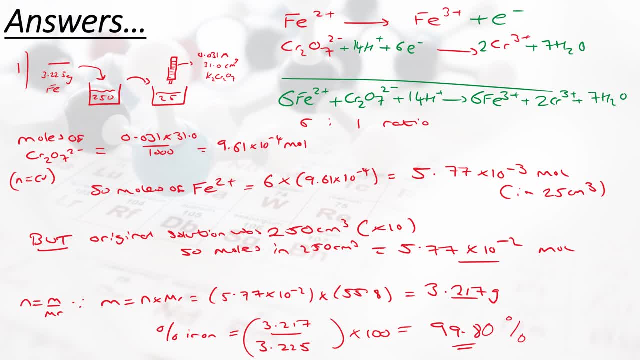 And of course that's actually what we want. We want the percentage of iron in the tablets, We want to work out the mass of the iron, So we need our moles of the Fe2 plus. So we now essentially just use the mole ratios here. 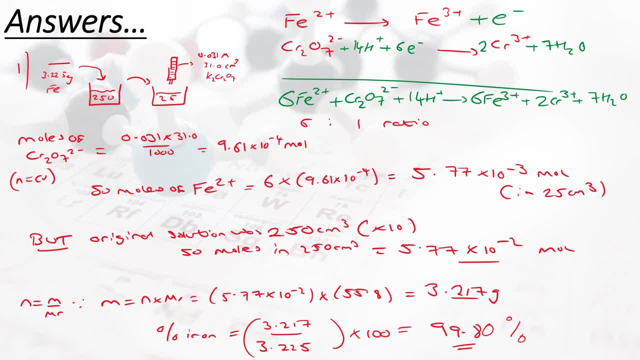 1 mole of dichromate is 6 moles of iron. So therefore 6 times that mole value gives you 5.77. Times 10 to the minus 3 moles. We then have to consider the volume that this is in. 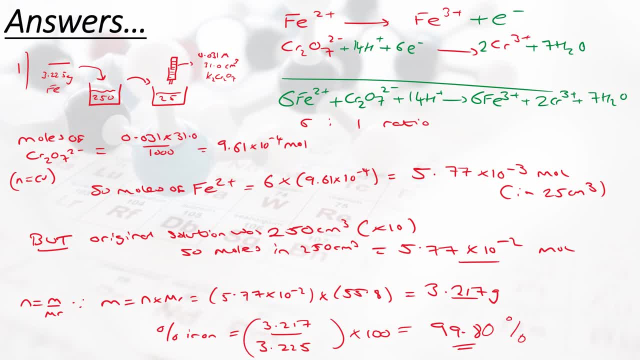 This is all to do with the titration that we've done, which was in 25 centimetres cubed. We want the mass of the iron that was dissolved up in our 250 centimetres cubed, So again we have a sort of 1 in 10 ratio here. 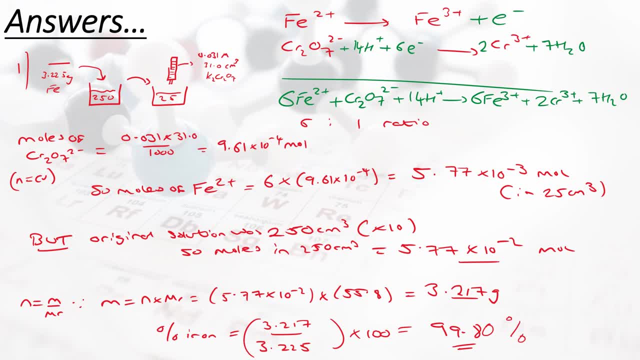 We've taken out a tenth of this for using the titration, So our stock solution is 10 times the amount we've used for our titration, And so the moles in the stock solution will be 10 times the amount that we have for our titration as well.